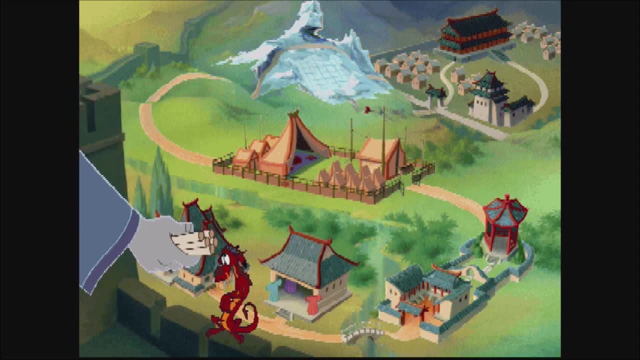 take them to the Imperial City and deliver them to the Emperor. He will spread the. Is that George Takei? the farthest corners of the Empire? Well, George Takei was in the movie, so the magic may fall out. 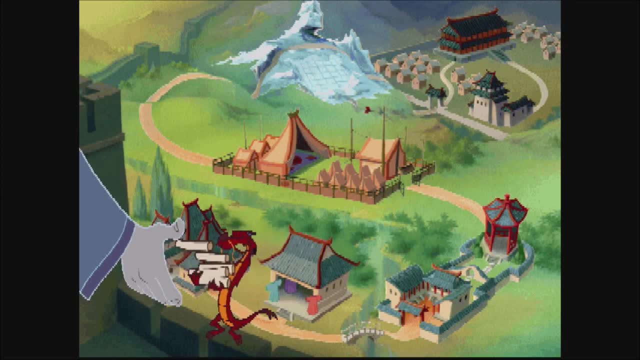 Hey, I've got everything under control, So it seems that we're playing as Mushu in the in this game. actually, Kinda, yeah, Now don't drop them Mushu. Okay, are we sure this isn't Eddie Murphy coming back? 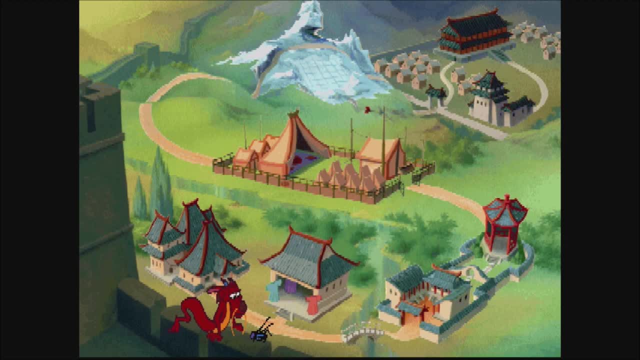 Because he sounds very on point as well. Oh, is it? Maybe Persian Vesa, Go ahead and check, Maybe, if they did get Eddie Murphy for this one. that's impressive, considering Eddie Murphy never returned for anything. Okay, okay, okay. 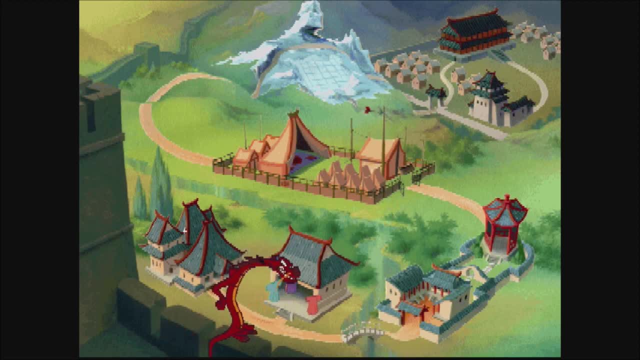 How powerful was that drop? if Mushu was able to scatter those scrolls all across pretty much the entirety of China, given the map, It's insane. You really needed a story, guys, because for some reason they couldn't tell the story of the movie. 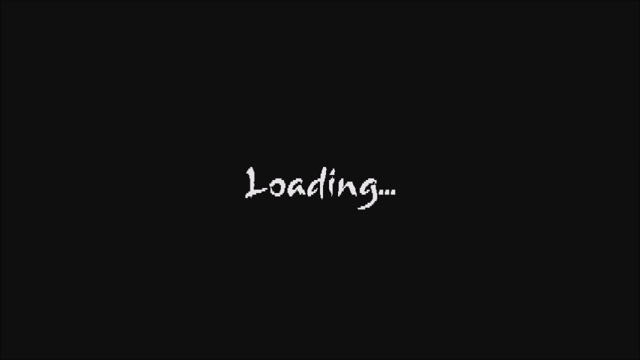 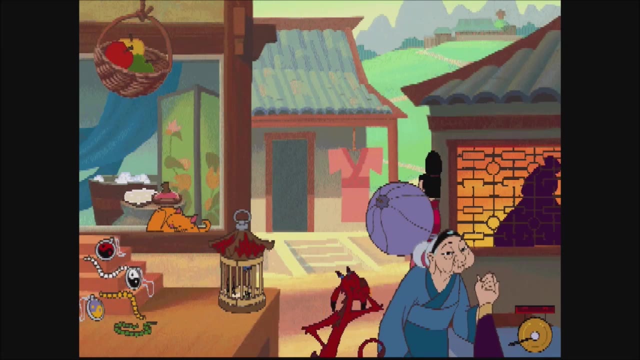 It is not Eddie Murphy, it's Mark Mosley, What she always said. It's so weird because we still do tell the story of the movie. What an excuse for having this omniscient figure that is the player to actually follow around. 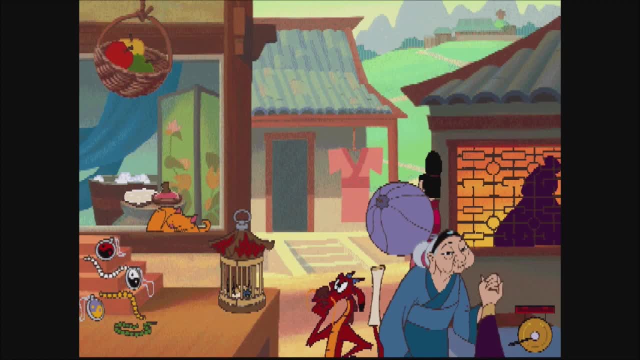 So essentially, we need the scrolls to help the plot happen. if I recall correctly, Yeah, basically. Okay, so He's arm wrestling. So yeah, This is a put and click, Put and click adventure game, except it's done for that preschool crowd, basically. 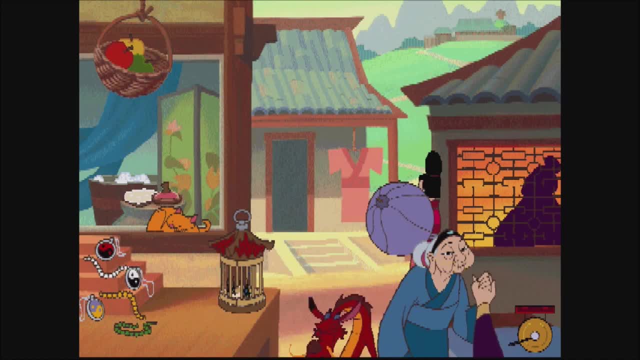 So it's not like a King's Quest game. Instead, it's very typical. You just click on things and it's The game pretty much tells you outright what you have to do. Also just to make: Sorry, go on. 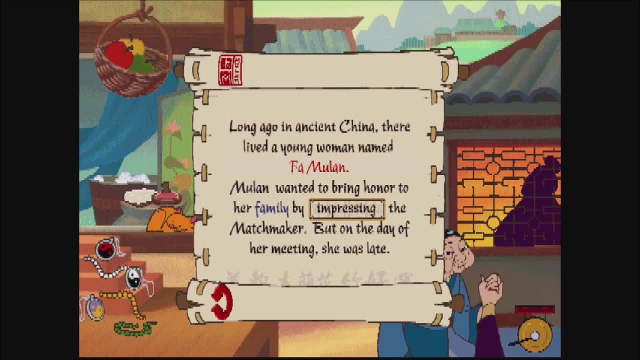 No, no, go on. Just to mention, the ancestor was not George of the Gates, that was Wells, according to them. Okay, We're talking about for the game of the movie. So yeah, Those who remember Game of the Gates of Prince of the Castle. 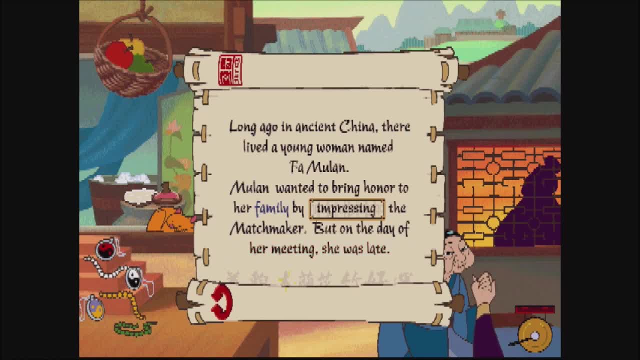 Because I'm pretty sure George Takei played him in the movie. So yeah, You have these things where the game tests your knowledge of the movie. So Mulan wanted to bring honor to her family by impressing the matchmaker, supposedly. 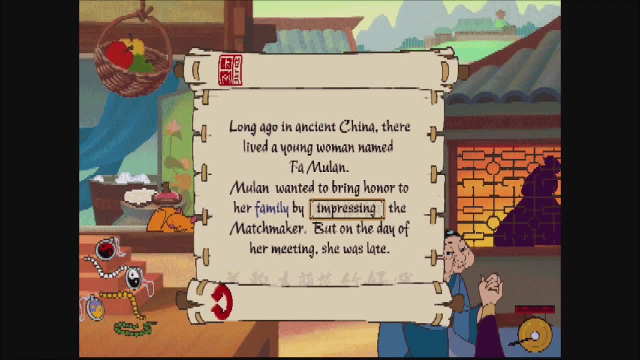 But the game also gives you a chance to pick another word. That being said, yeah, It would be impressing. So kind of interesting. I'm going to struggle. Essentially, what Amazing is up with this game is essentially the plot is that you get scrolls that are retelling. 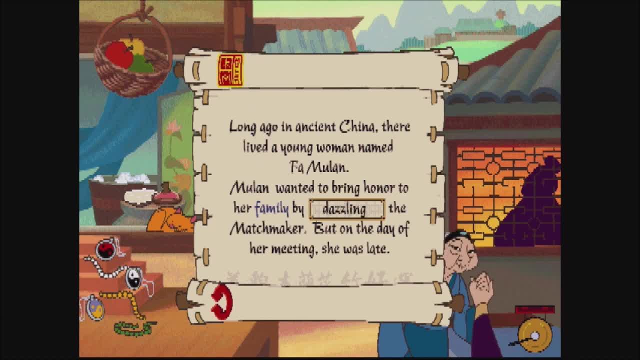 the events in the movie, if I understand correctly Basically. If I understand correctly Basically, yeah, By dazzling the matchmaker. Let's see. Hmm, I would normally go with impressing, but let's leave it dazzling. Mulan wanted to bring honor to her family by dazzling the matchmaker. 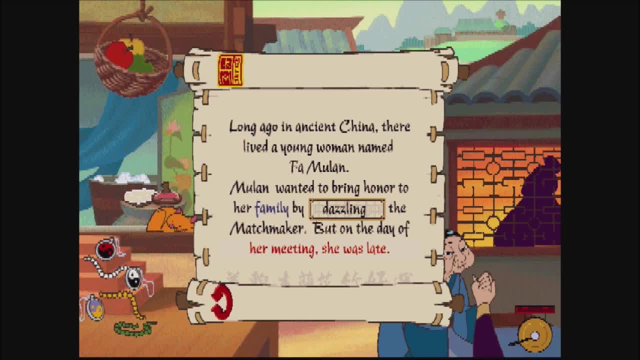 But on the day of her meeting she was late. Hmm, Okay, That doesn't. Yes, Dazzling- That's how I read it. I mean dazzling and impressive boils down to the same thing, but whatever Amazing could work. but I think it's been the wrong tag. 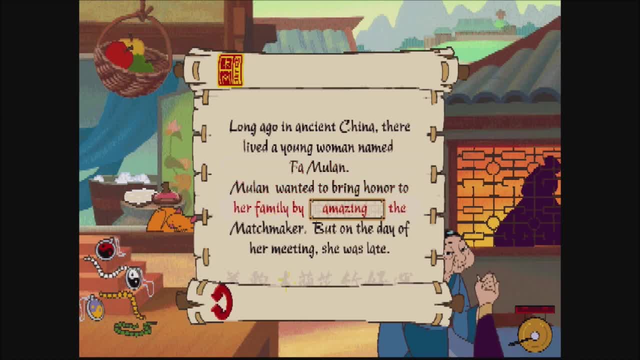 Sure, This is actually one that you grew up with, So want to talk about it. On the day of her meeting she was late, I'm not sure how. Yeah, that's the thing I can support, because actually me and my sister actually also played this when we were kids. 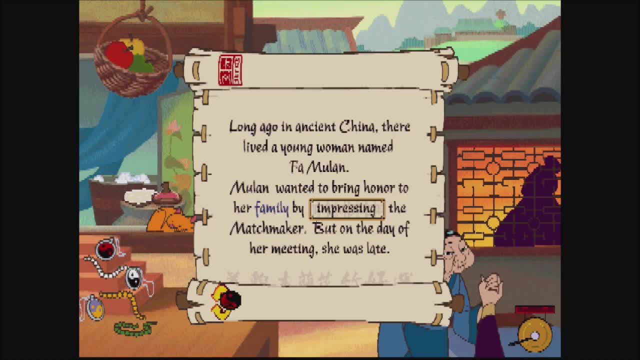 Go on. It's very short, but I enjoyed it. Keep in mind it was a bit before my mother introduced me to King's Quest, So as far as point-and-click games was, this was technically one of my early experiences. 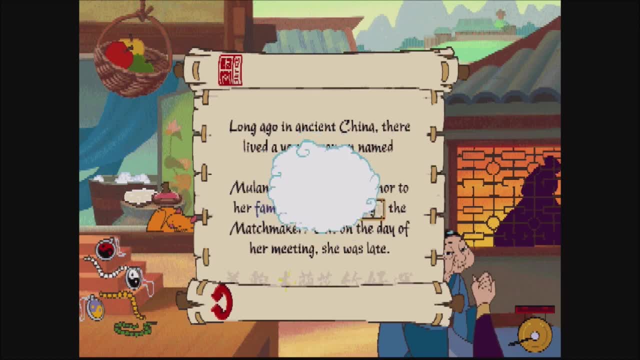 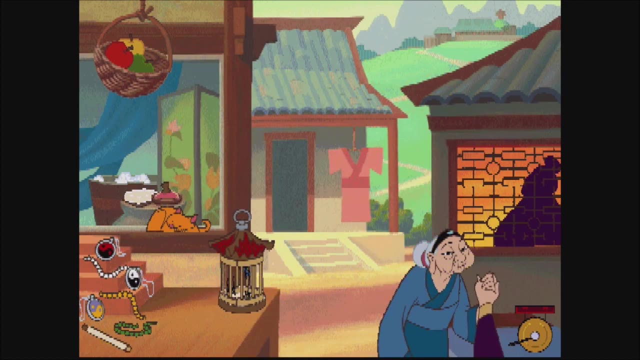 Yeah, there you go. Yes, it's also being a very early experience for me and my brother, because I had mentioned before that I basically grew up on licensed games. Mm-hmm, Um. for me, my My history with this game goes down to this. 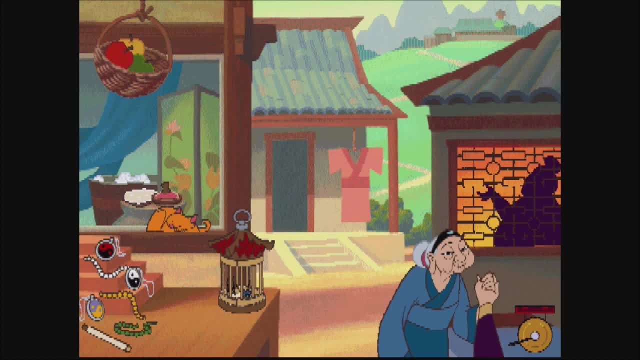 One day I saw in the store shelves: oh great, they made a Mulan game for the PS1.. Let me see, And I looked at it- oh, it's not a cool action platformer where I go through the sections. 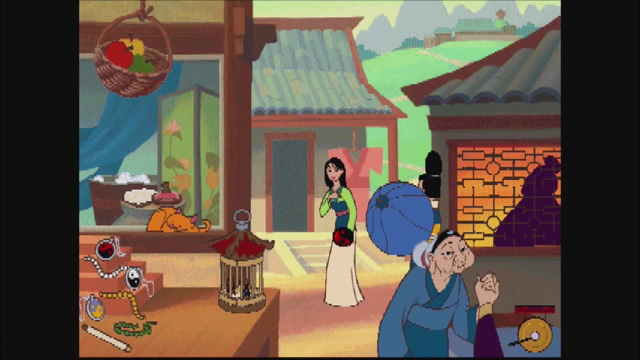 of the action bits of the movie and shit like that, like the other Disney games, So I kind of like. So I've always felt that Mulan is one of my favorite movies from the 90s Man, there's movies everywhere. 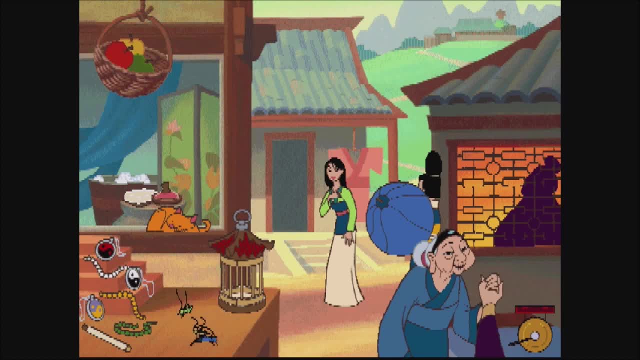 Um, And I've always felt it was such a missed opportunity to not make a more typical Disney action game like the other movies got you know, Because Mulan is so perfect for a game, For the kind of game we were getting like with Simba's Mighty Adventure and stuff like. 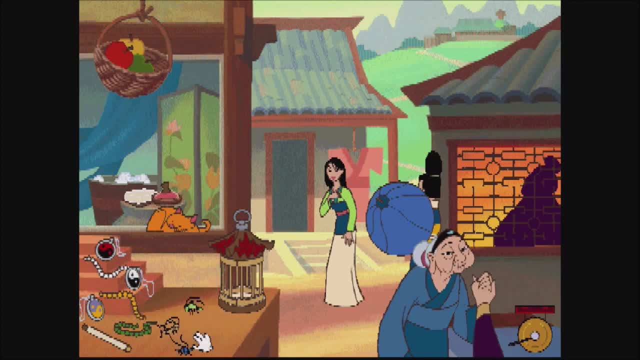 that you know, Like I'm still kind of really puzzled that they never got around to making stuff like that, because this movie practically begged for it. I mean, there's so many cool action set pieces in the movie that would lend perfectly to. 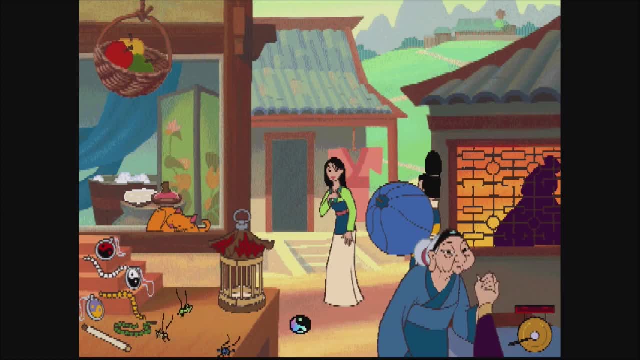 video game levels Boy. she sure is picky. Considering how kind of they wasted them for the themed world in Kingdom Hearts 2 as well, I get the idea Disney Interactive might have not had much. Remember, Joe, most of the world is just a giant escort mission. 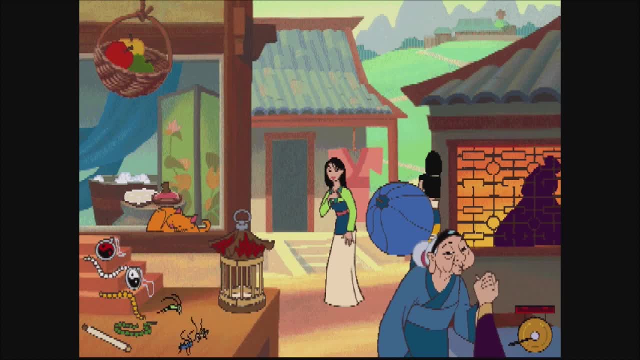 The Avalanche set piece is laughable for how it looks. The only good thing is probably the fight against the Shan Yu at the end. basically, Yeah, I want to. I would say that Mulan had good enough rep in Kingdom Hearts 2, but I do kind of miss them. 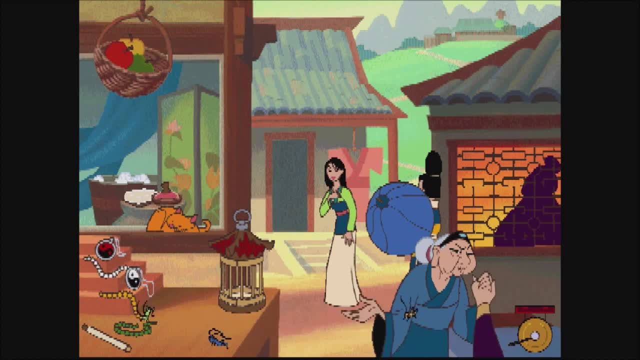 kind of get your point. I could have been. yeah, anyway, yes, trips, I want. I wanted to have a bit where you could dance along to I'll make a bad out of you. well then, the next screen is kind okay, not kind of, but not really that. it's weird, you'll. 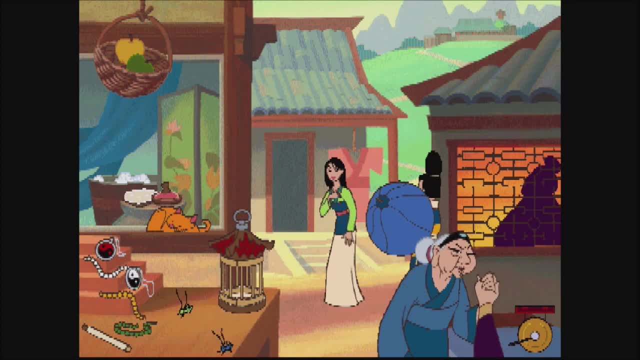 see, let's give an apple to grandma. so well, okay, so are we essentially, or does this game take place after? yes, no, no, you'll notice. M1 is now about to go get ready to meet the matchmaker. we can move forward. see the thing about this game. 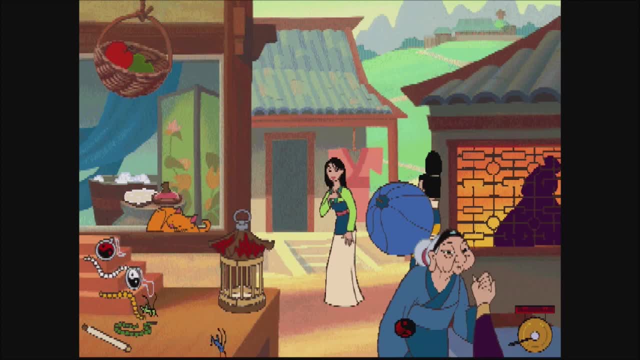 job is that you don't necessarily have to complete anything. you can just press the app of the up arrow on the door to move to the next screen. thing is: if you do, if I just skip everything, the game would be over in a minute. so I'm trying. 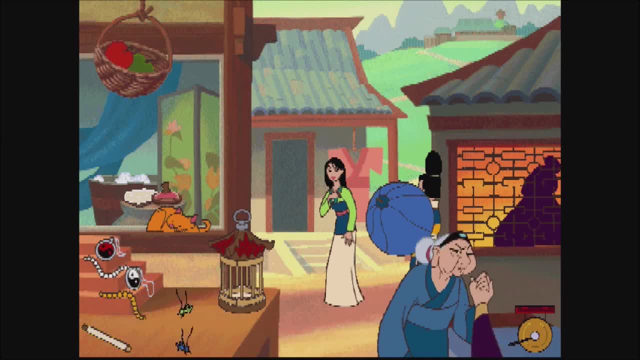 to click on. so basically put this was down to this job, but click on video and then click on the next video, and then click on the next video, and then various things to see what does what, and when you get bored of this screen, move, move to the next one. that's basically the game and sadly there is no. 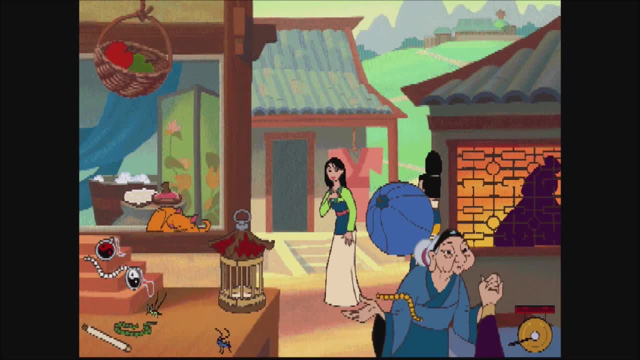 real challenge, because if you fuck up, let me just tell you no, I don't want this, and you know you're just have to pick something else again. you can tell me this game, this game, this series of games, was done for very young children. yes, you're right. yeah, because, as you can like, probably here, grandma over here is. 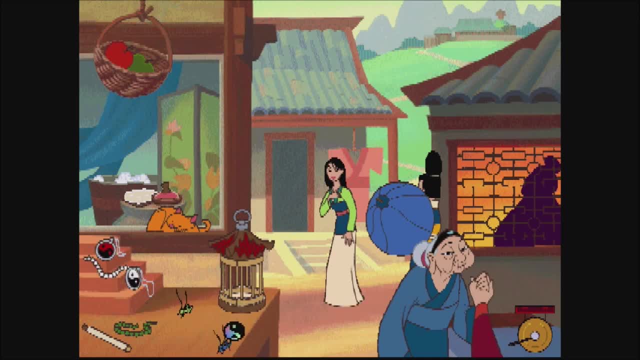 telling you exactly the thing that she wants? yeah, not even a hint. it's like no, that one, you did this game, but this game ever get to our language version doors? just English, yeah, I can, much like I was. much like I cannot speak for every other us or things about that. much like the. 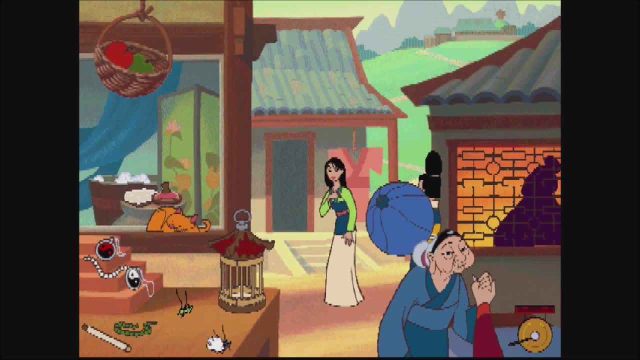 vast majority of these interacting games a deep gallon tarp. localization: perdu, apple, my country, sadly. I'm liking for the English which is, it usually meant, a very. we could not bring the actual list, check those for the game, for the movies, because they tend to have a lot of. 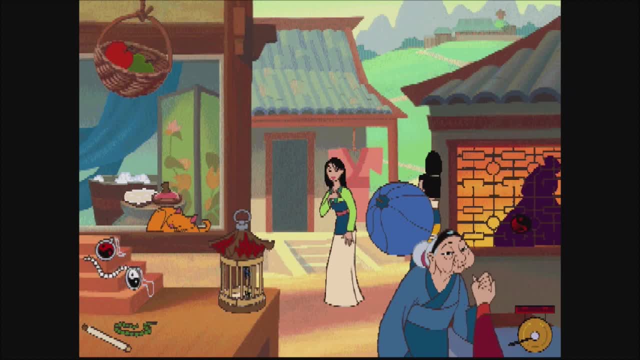 celebrity cast that normally don't do video games because they think they're just kiddie shit. Oh my god, is that still a thing over in some of those countries? If I had to talk about how bizarre the industry of voice acting in my country will be. 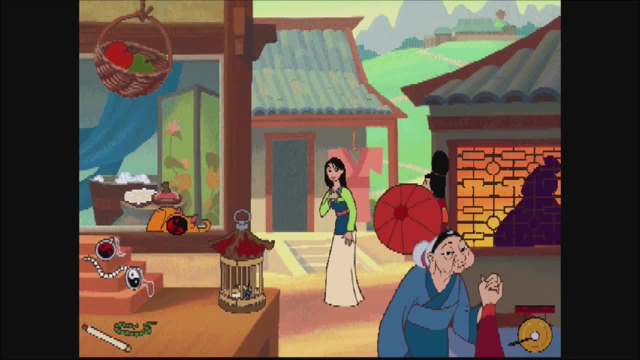 Anyway, now to give this game some credit. while it's not the most exciting game, this is a game that fulfills a certain niche of games that I can appreciate. You know, I mean obviously now grown up, these games aren't as much. 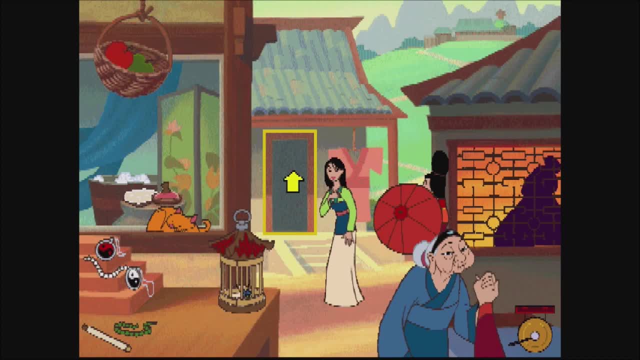 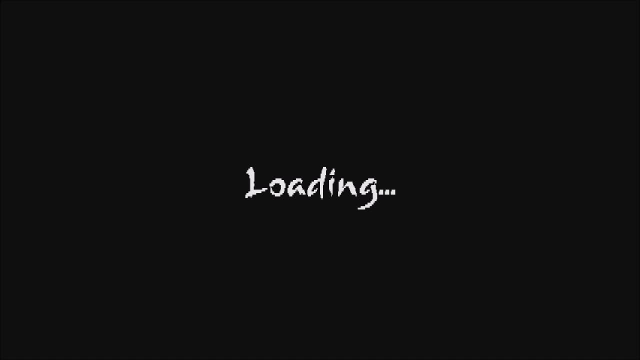 my speed, but these are definitely the kind of games that are perfect for kids who want to try to get into gaming but really are incredibly newbie to it. And yeah, the load times, as you can see, unlike the PC version, the load times on the PS1 version. 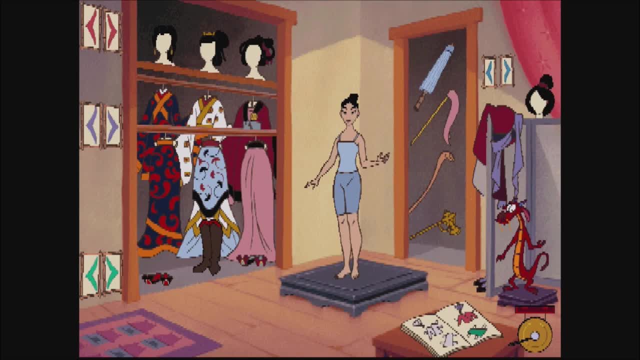 are quite longer. Oh boy, dress-up game Also. I'll be honest, I don't think. I think they woke poor Ming-Na up from her sleep when recording this game. Are we sure? that's even Ming-Na Wen again? 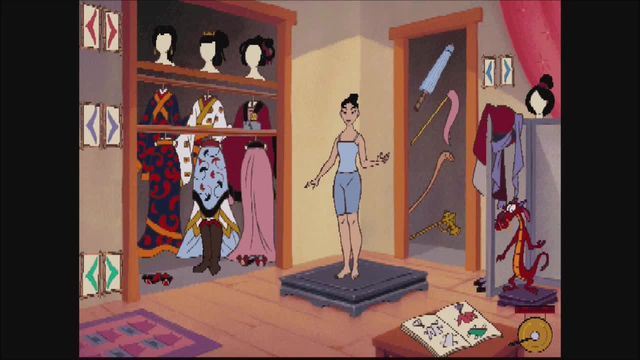 for this game. Yes, it is. I can recognize her voice. She is very loyal to this franchise. I mean, Ming-Na has done Mulan in pretty much literally everything, as far as I'm aware, hasn't she? 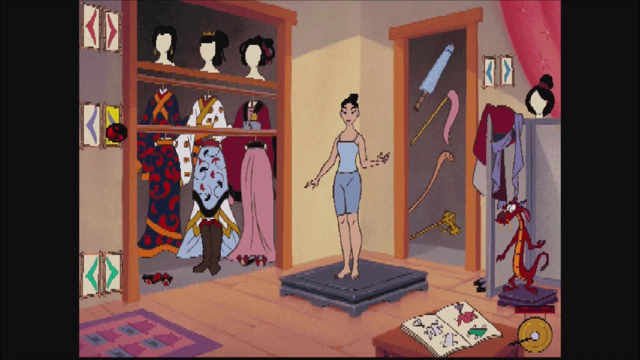 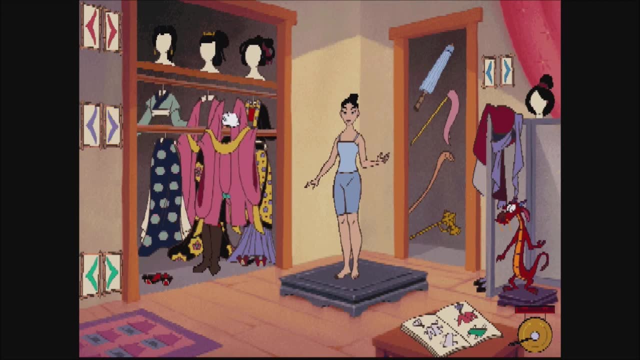 I don't think there's ever been any sound-alikes for her. I mean, she even cameoed in the shitty live-action remake and everything. so Yeah, Let me see. Yep, yep, she was in Kingdom Hearts 2.. Yeah, of course I think most of them were. I think the only ones who got recasted were the Emperor and Shan Yu. I don't even remember who voiced Shan Yu in the original movie because he has so little lines. Well, I remember that in. 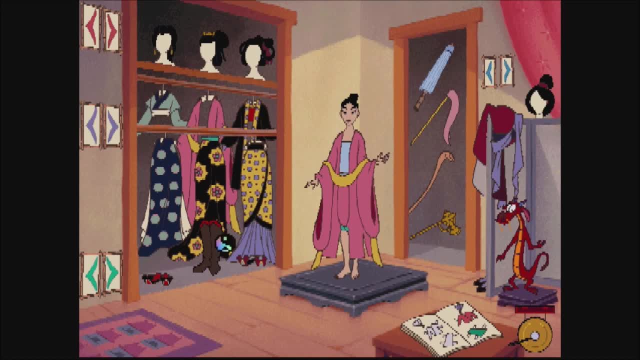 the in the original film the Emperor is without Pat Morita, aka Mr Miyagi from the Karate Kid movies. Yeah, Which does apparently reprise the role for this? Indeed, Oh, it's interesting. 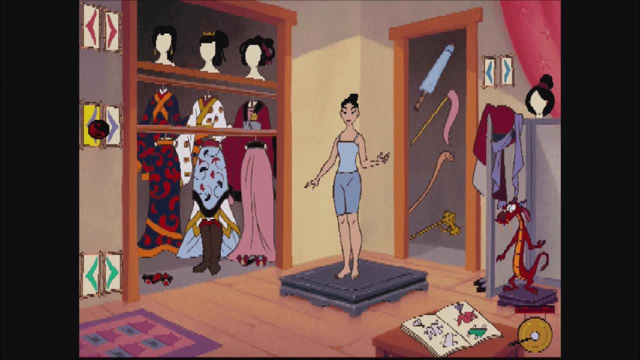 Well, if it helps you to like my country's dub, got one of our best voice actors to voice Shang, specifically the voice actor who's very well known for playing the main character in Rainy Rukin Shin. So there you go. 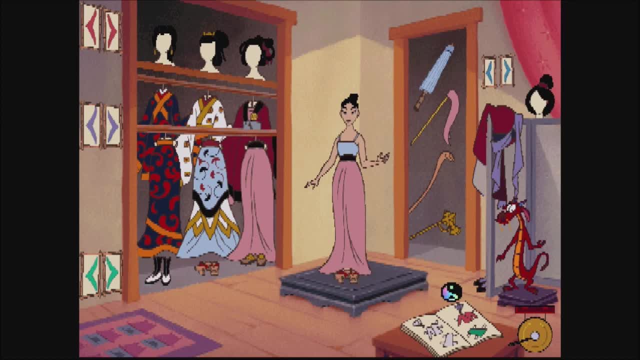 So he's used to playing those kinds of characters. Yeah, basically get the right outfit. That being said, you don't actually have. Once again, you don't actually have. The game is incredibly forgiving, and by forgiving I mean. 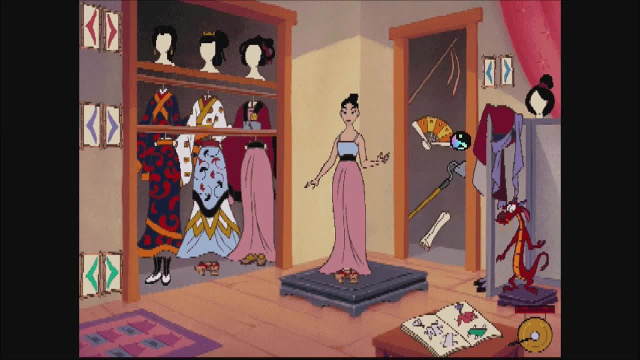 the challenge is exactly zero. The game doesn't demand that you get the outfit exactly like in the movie. Instead, just dress however you want and then move on when you're tired of trying various things. See kids. Now you can imagine the movie. however. 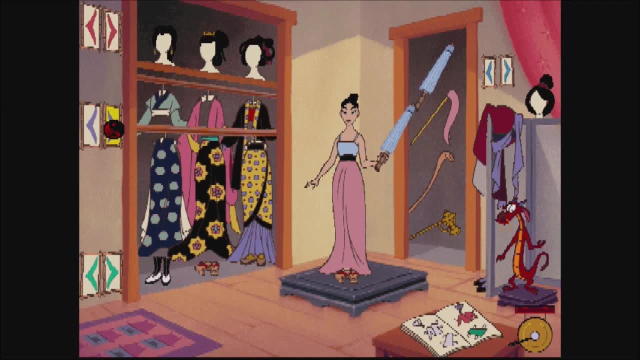 which way you want it Basically. yeah, I might as well. You can even give her wigs too. Yeah. while this is going on, I actually want to bring up something that me and Shiroi actually had a disagreement upon at the end of our Pocahontas run. 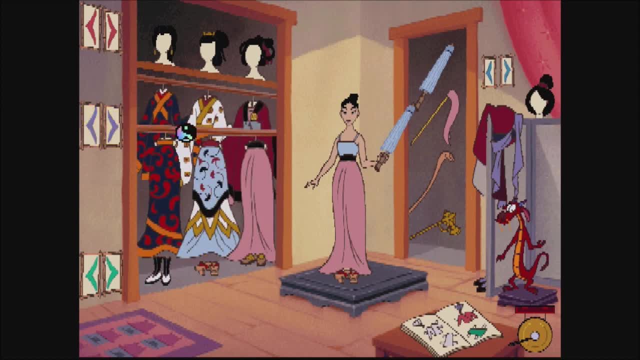 where Shiroi wasn't particularly impressed with the Pocahontas game and she felt that the storybook direction would have been a better case, where I think I I disagree. I feel like they did a good job drawing gameplay out of the limited potential. 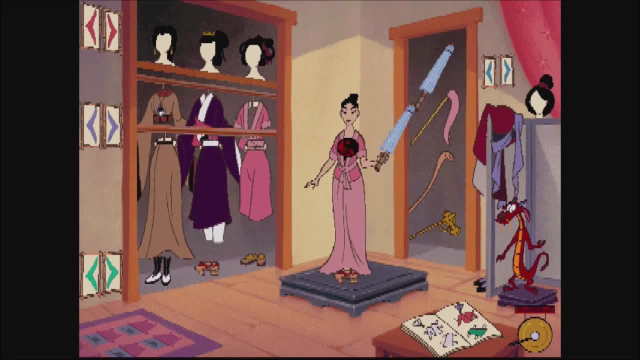 that Yeah movie had, Whereas with this game, again, I have nothing For the record. I have nothing against this game existing. It's just that the fact that this game, despite being much better, much easier to adapt into a video game. 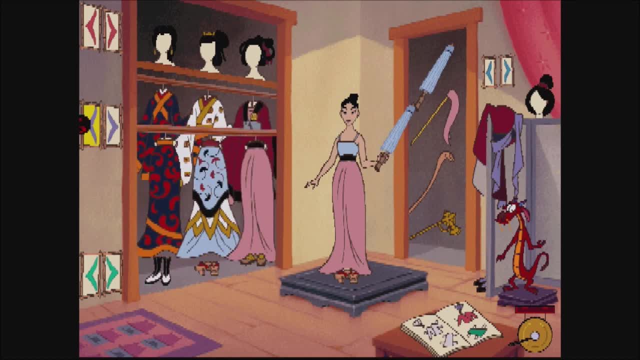 didn't get a proper action video game out of it, like Hercules or Simba's Mighty Adventure, still kind of irks me to this day because, God, what a missed opportunity. Imagine a PS1 game where you're having a cool action level. 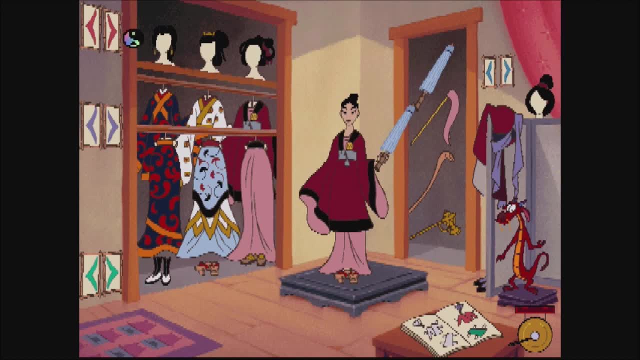 where you're trying to survive the avalanche or something like that. you know, I love how they literally have Jafar's staff as one of the things you can pick, Yeah. So basically the Aladdin movie was like the real ending was that she killed Jafar. 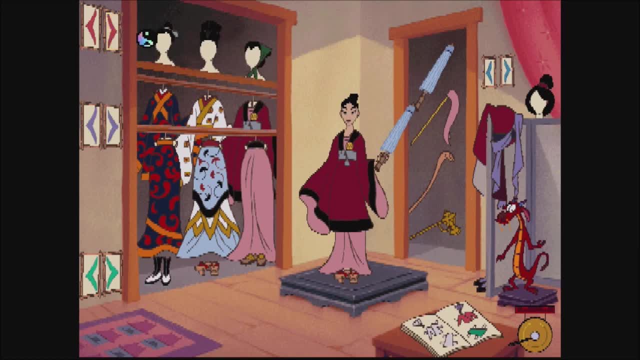 Probably Jova Jova. probably because they still had the sprites that they made for the Aladdin-David Perry game lying around, because, remember, this is one of the last games to have Disney Animation. do the sprites. So in the animation. 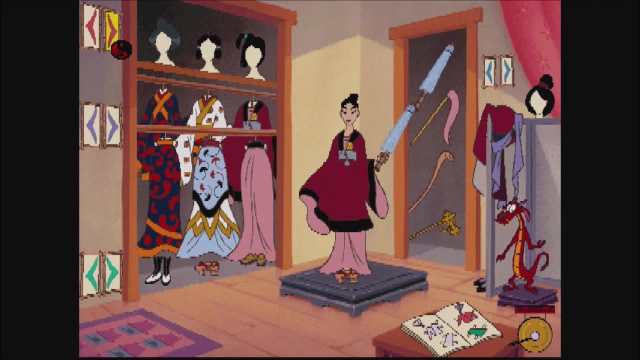 of the sprites, So probably Go on. Is that staff the same sprite from the game? It looks a bit clearer, but maybe they just patched it up. In terms of these storybook games, the one I remember the most is playing the Lion King. 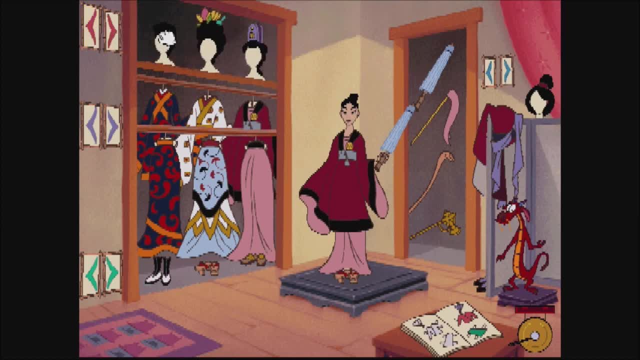 on PC. I can help you there. Jova, Before Mulan was a thing, Disney Animation Florida, because remember this was back in the day where Disney Animation had multiple studios over the course of the US Instead of just one concentrated big studio like they have today. 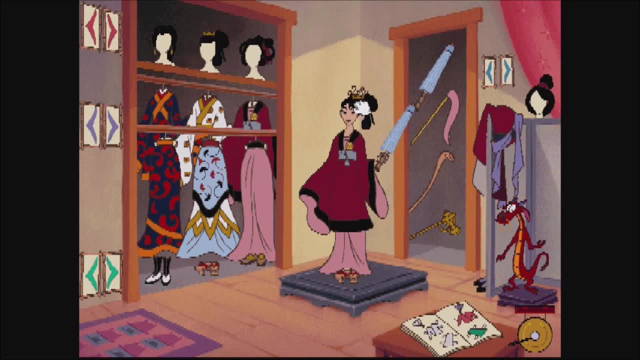 Back then, Jova, back in the early 90s, it was Disney Animation Florida who was in charge of doing the animation for these video games, whereas the proper studio in California would be the one to handle the movies and stuff like that. 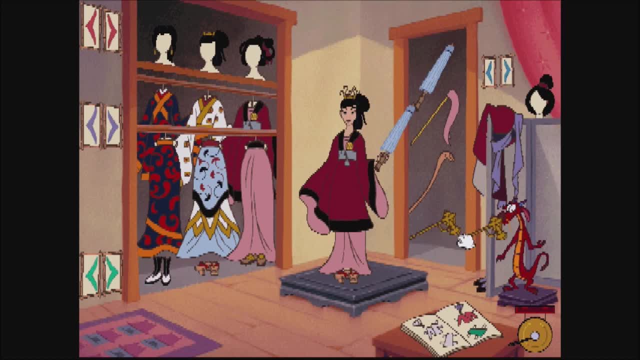 However, by the time it got to the mid-90s, Disney Animation Florida was given a chance to make their own movie, and that was Mulan. So my guess, Jova, is they went straight from making Mulan to making this game. 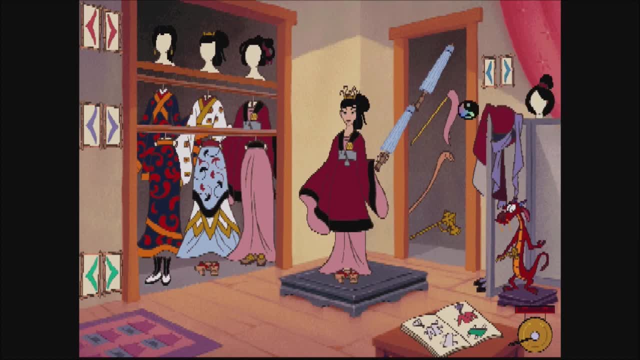 I mean Interesting, Also considering what you said with the tour series. well, apparently, as far as this series of games is concerned, there is one about Pocahontas, so maybe we should check that out. Oh, I'm sure there is. 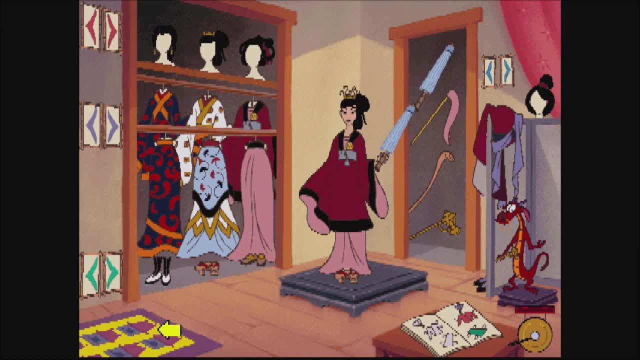 You know, the main reason why I'm doing this one is because it's the only Mulan game that exists, except for that bootleg Chinese one. So Wasn't there one for the Game Boy Advance, Was it? Yeah, give it a call actually. 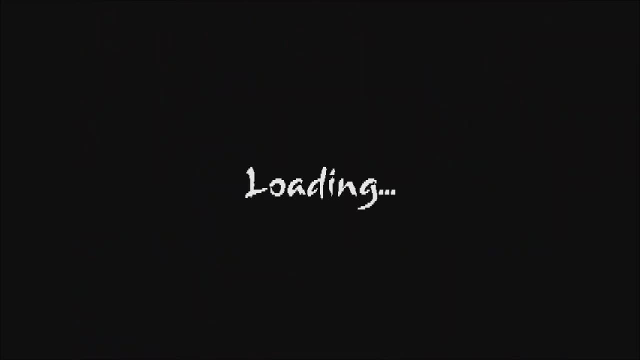 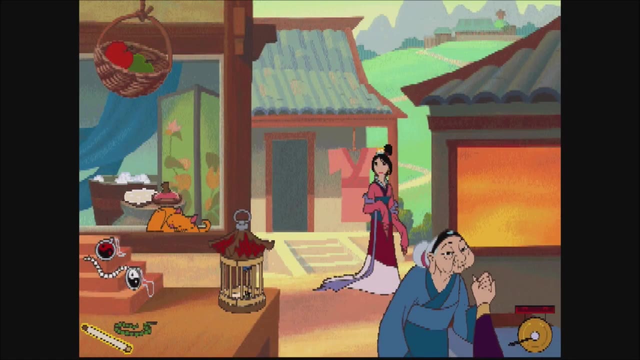 There's one on the Game Boy. On the Game Boy. I'll have to look at it. I think, considering the console, it's probably not that great. Is there any info? Go on, Shira. Is there any info out there? 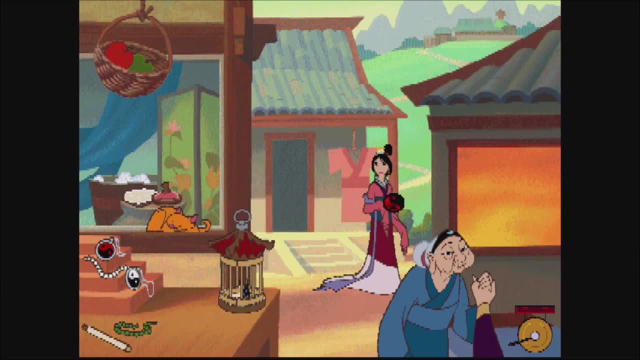 about why they took this approach. Well, remember Shira. the reason this game exists is because, again, there was this entire big series of storybook games that Disney was making regardless of any other video games, Because, remember, Pocahontas got both that game. 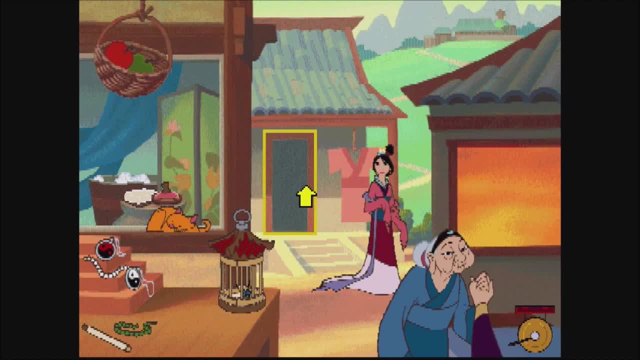 we commented on, as well as its own storybook game. The thing with this is that this game only got a storybook game instead of getting another video game that's more console-oriented, rather than Because this is a PC port. Remember, this is a port. 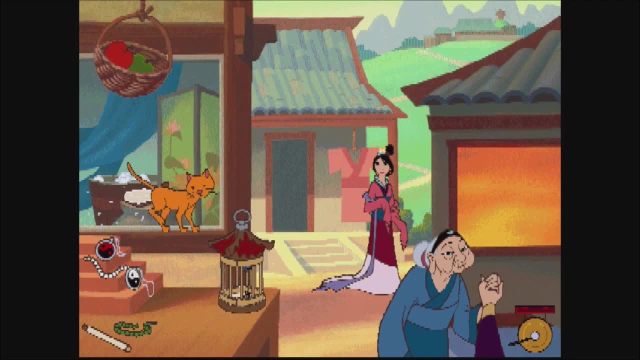 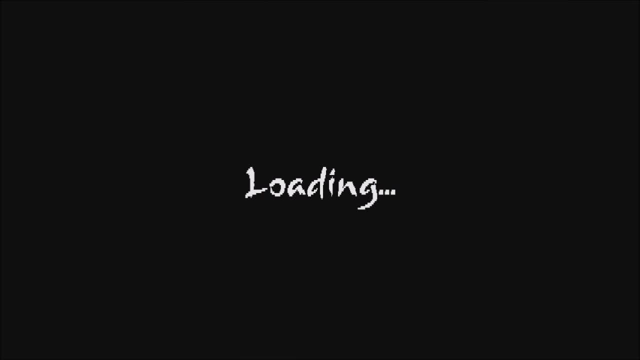 from a PC version. So go on, Jova. I'll admit I did that probably a little often, just because it's funny. Oh yeah, no. As for the storybook game craze, here I can sort of get. 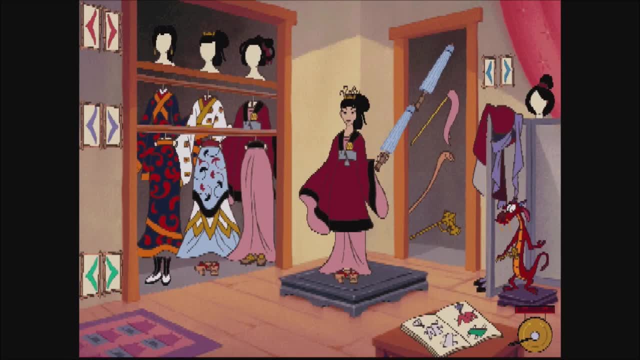 why those were in the vogue at the time. One, they were a great way to show off some of the advanced gaming technology of the time here, Ergo, getting something like a movie-like experience. Yeah, believe it or not when you think about it. 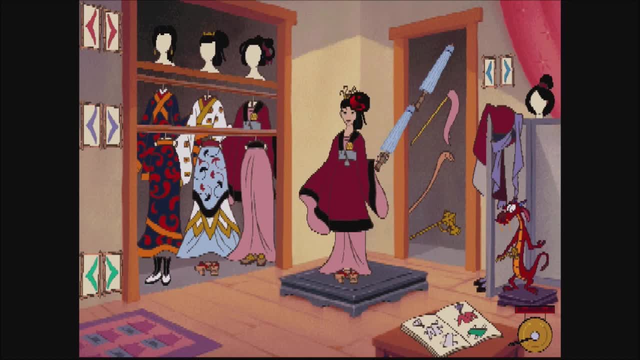 storybook games were kind of the cinematic experiences of their time Two. they were incredibly simplistic gameplay-wise, which meant that they could reach a very wide audience, not just in you know backgrounds or taste, but, of course, in ages. 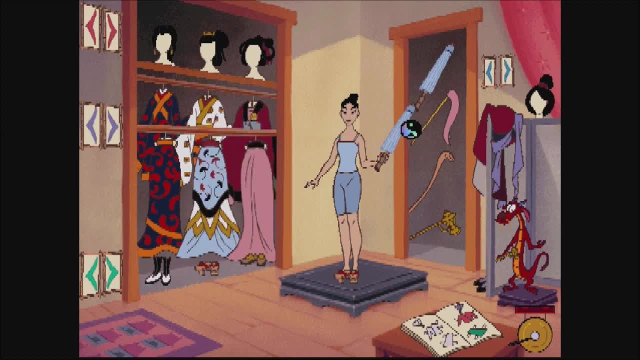 So again, ironically, I feel like getting this game as a storybook thing probably would have been seen as a great honor back in the day. Oh sure, Granted And granted. maybe that Game Boy Color game was what they thought. 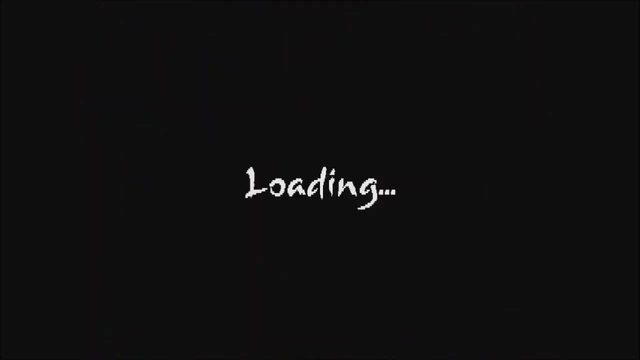 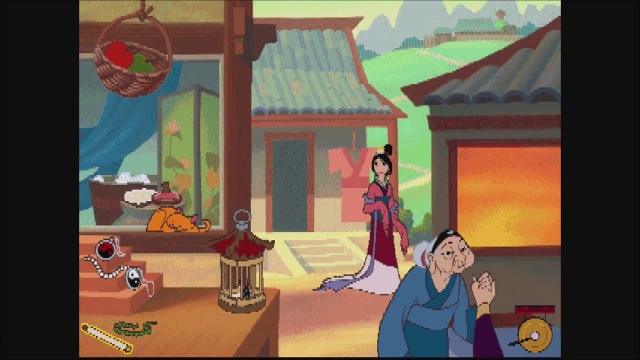 okay, that can suffice as the action one, assuming that that's a thing overall, Because, yeah, there was a time where handhelds were considered pretty much. oh, you know, they can pretty much suffice as the main game, especially given how Nintendo. 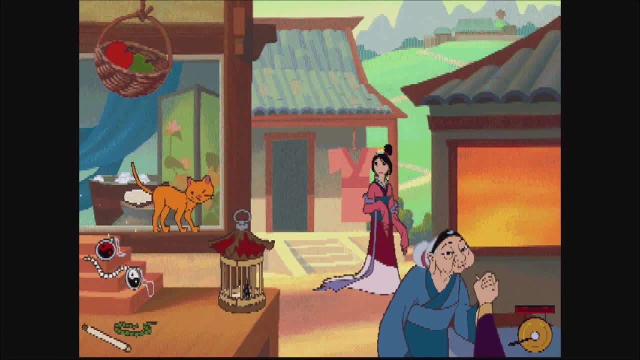 were absolute juggernauts with their handhelds. So to some companies, having a handheld version was pretty much just fine in and of itself. Basically, You'll also notice that regardless of how you dress Mulan, she'll always have the movie outfit. 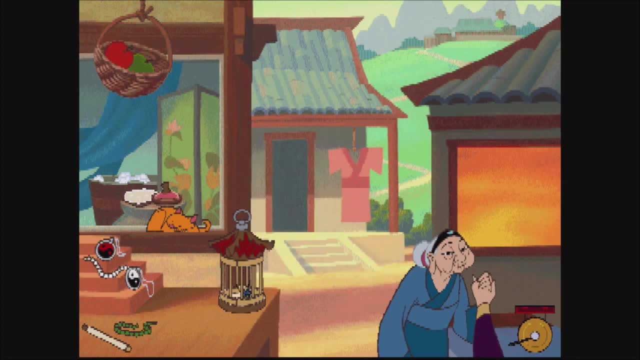 in this screen. So, yeah, it doesn't matter. Oh yeah, and you can still take a bath, even though you're supposed to already. Yeah, you can basically screw up the order of the events by having Mulan take a bath. 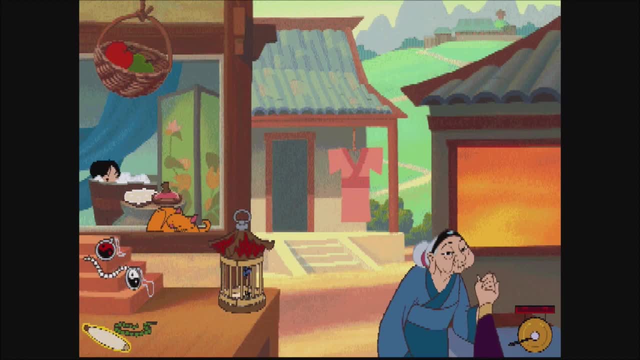 after dressing for the matchmaker. Could you imagine if you could do that for the whole movie? You could put the end at the beginning. Also, what Jovo was saying, it's at least partially also true, because, if you forgot, Disney had a couple of early. 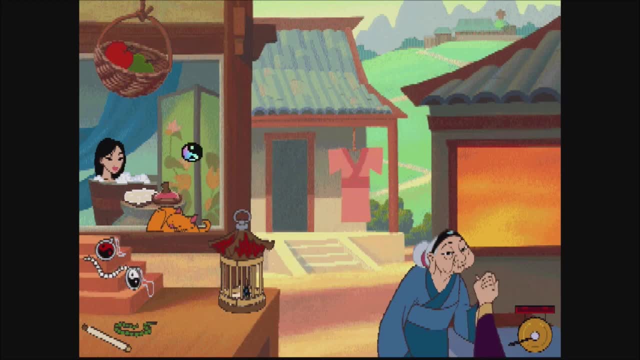 point-and-click titles back in the older days, For example, one based on Winnie the Pooh and the Unbreakable Woods by 1985, and one based on The Black Cauldron- And because of the process that they had. 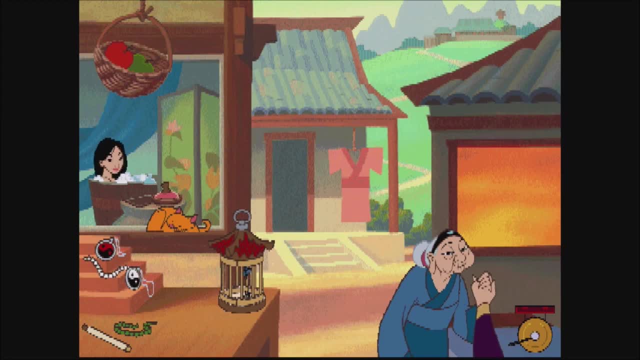 apparently it was a good idea to exploit it. Like I said, they did. actually a lot of them Again. there's one about Lightning, two about Winnie the Pooh, one about Pocahontas. Toy Story, Dungeons of Redemption. 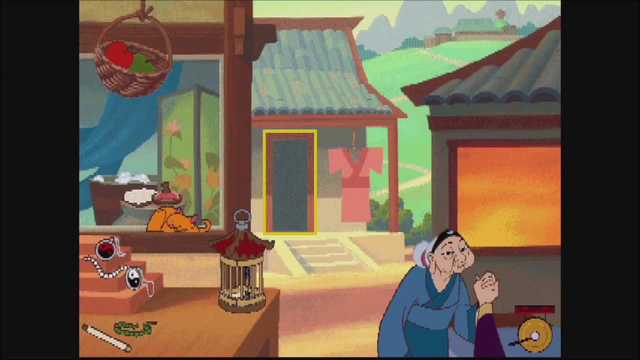 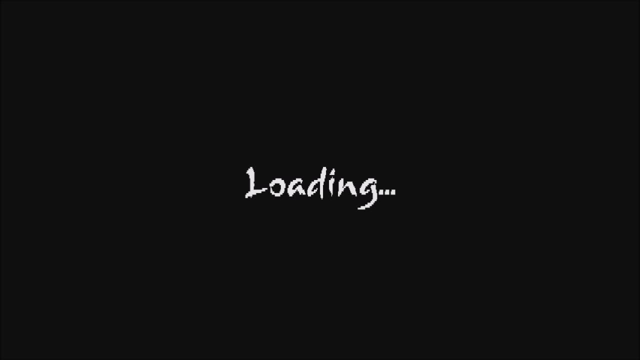 One about Mace, Hercules, Little Mermaid and this, So there's actually quite a lot. Sure, Wait, Mulan, you changed back into your regular outfit Because reasons I get that. It's just that the fact that I had to wait. until 2006 to finally have a boss battle against Sean Yu kind of still irks me. I mean, to be fair, it's probably even more what happens in the actual movie anyway. Ouch, But he's right, Um, granted. 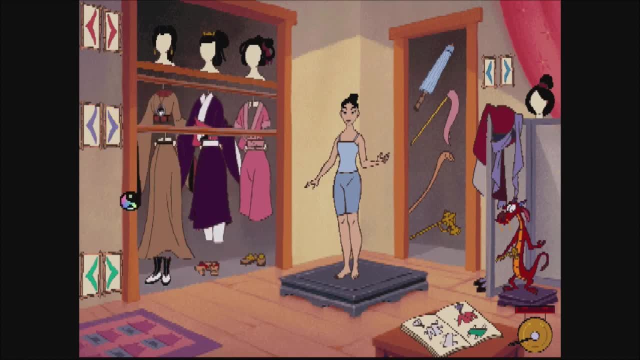 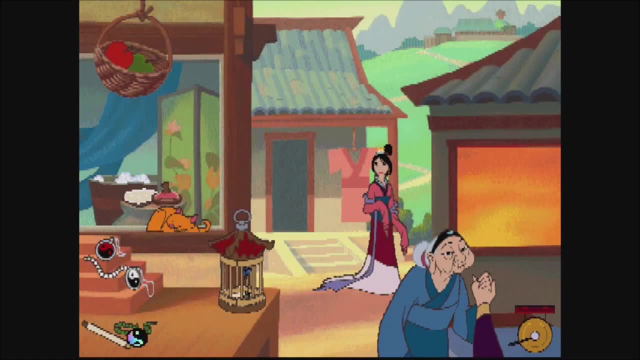 Hopefully. well, okay, If what Dwebs said about the Game Boy Car game is anything to go by, technically, you may not have had to have waited that long. Sure, sure Granted. okay, let me actually Google this to see if that Game Boy Car game 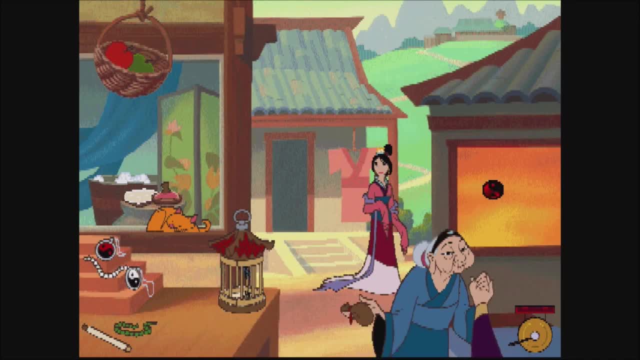 was a fan, Sure, Um yeah, that's the basic gist of it, And now she's giving you that shit. Go on. Yeah, Mulan did have a game on the Game Boy Color. Yeah, like I said, it's done by. 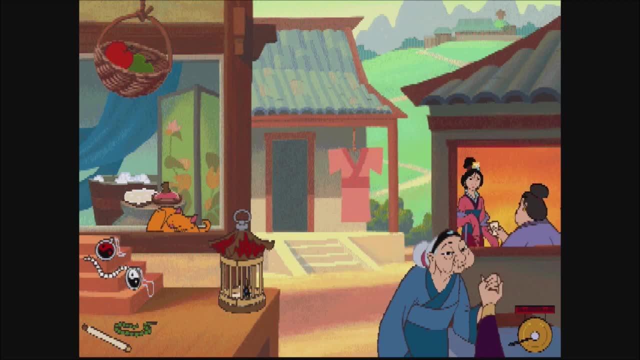 Oh, here we go. Matchmaker, Yes, Matchmaker. Thankfully, we were spared by the very painful comedy the Matchmaker was subjected to. Yeah, I like the comedy, but whatever, He is not as big a fan on the slapstick. 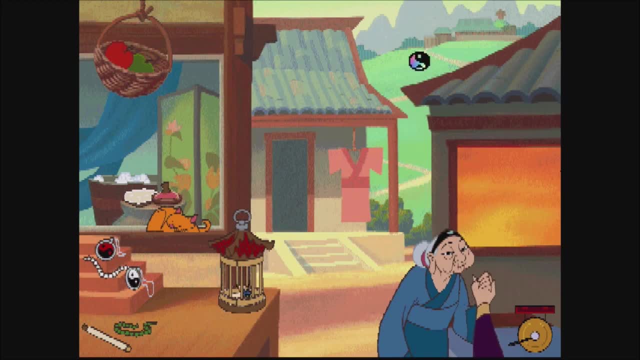 it seems. No, that depends. Some worked but some didn't, and it overstayed its welcome to me. I think it worked in there. That said, I do not care for how it was done in the live-action movie. Well, I love how. 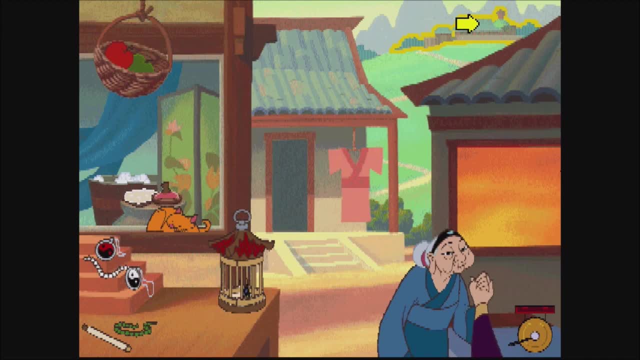 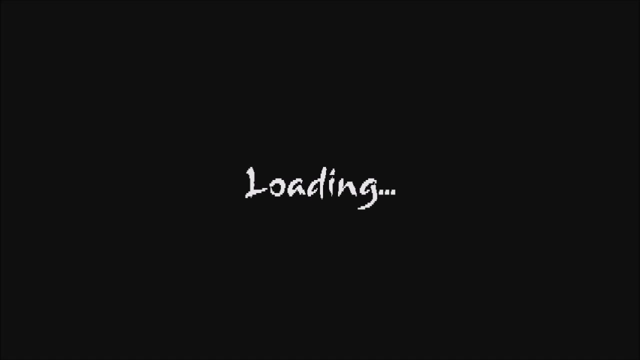 I love how this will take you to Mulan. It's an era of movies. I'd like that one really big thing that people keep bringing up, Like the statues in Hunchback, the comedy in Mulan A lot of people like. 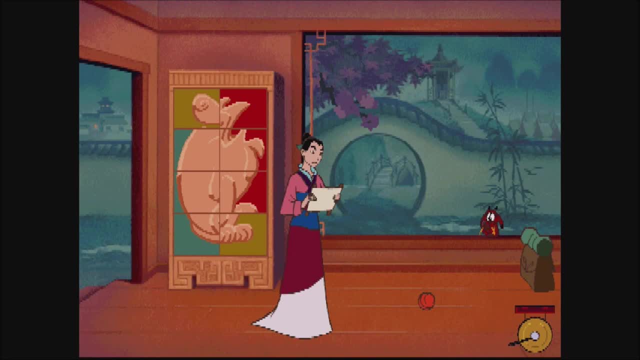 the comedy in Mulan. I mean, granted, some don't, but I never. no, I mean, okay, the comedy in Mulan was never, as it never got as much backlash as the gargoyles in Hunchback of Notre Dame. 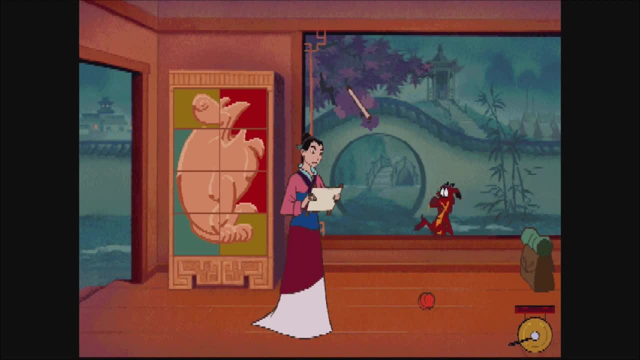 Honestly, the biggest complaint that I can say about Mulan is again that, despite having a big presence and a genuine threat to the Chinese empire, again that Shan Yu is probably one of the worst villains of this role of its time, Pretty much. 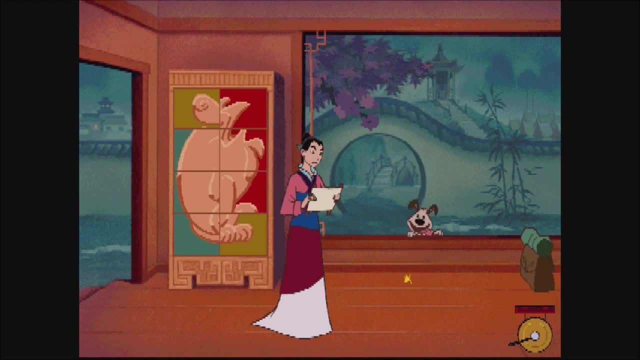 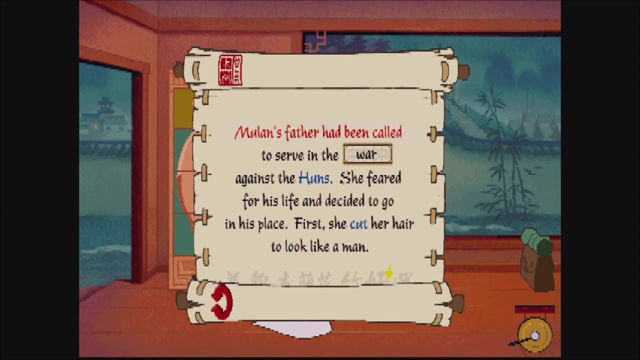 Like he's good and threatening but he lacks a lot of the presence and nuance that you know. that makes a lot of the Disney villains of the Renaissance beloved, And I get maybe that was their intent, I mean, I guess. 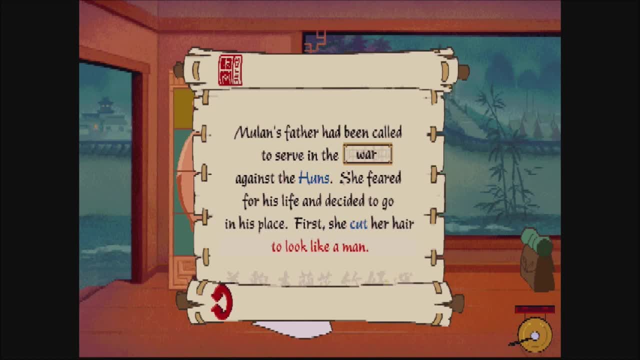 it does keep them from being the same as the Disney Renaissance films. Do we know about if development was actually, you know, troubled, similar to what happened to the King of the Suns, Because that would explain. maybe Shan Yu was supposed to have more screen time. 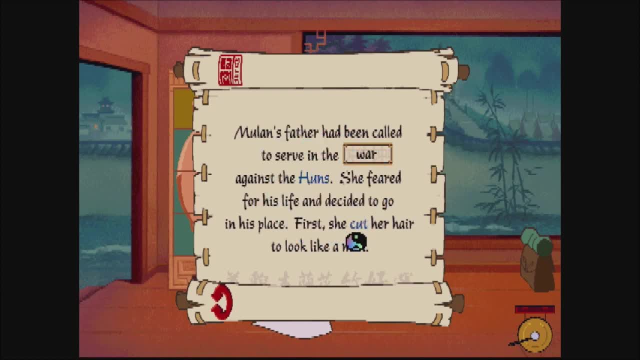 I don't know. I have not really heard anything that suggests that the Mulan movie was in any development hell. And yeah, if you're pressing any of the words that are highlighted as blue, you'll be able to see a little animation of it. 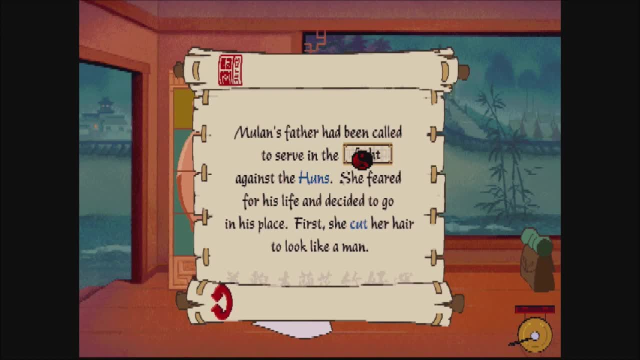 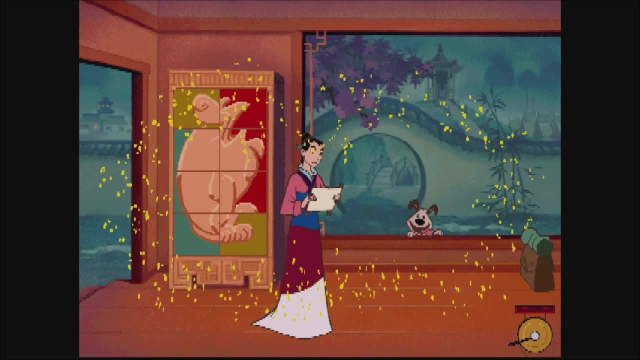 Yeah, here's another thing, by the way: Serve in the fight against the Huns, or battle against the Huns or war against the Huns? I mean, I figured all three of those words should technically work, but whatever, It's kind of weird. 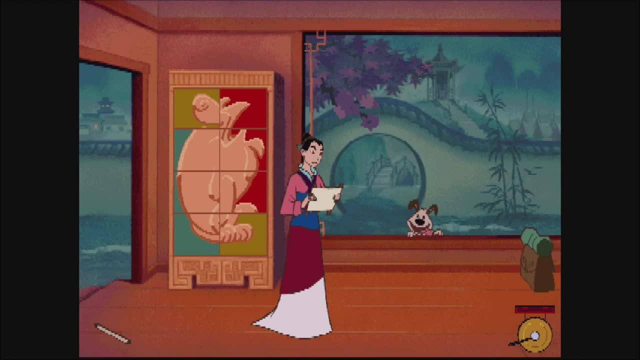 because you'd think they would have, especially because this is meant for preschoolers. you'd think they would have, like a word that is clearly the right one and two words that are clearly the wrong ones, because they don't even match the context at all. 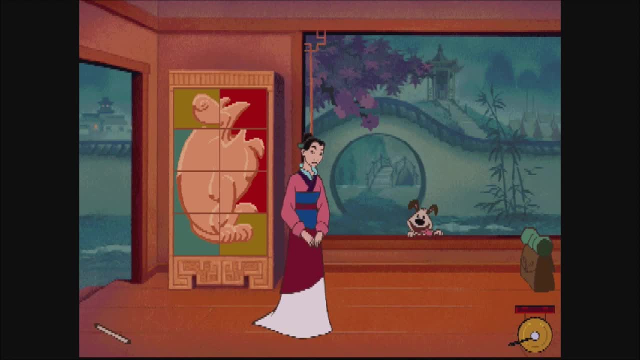 But instead they come up with three words that all really work when you get right down to it. I mean you could use. you can say: go to the war with the Huns. you can say, go to fight with the Huns. 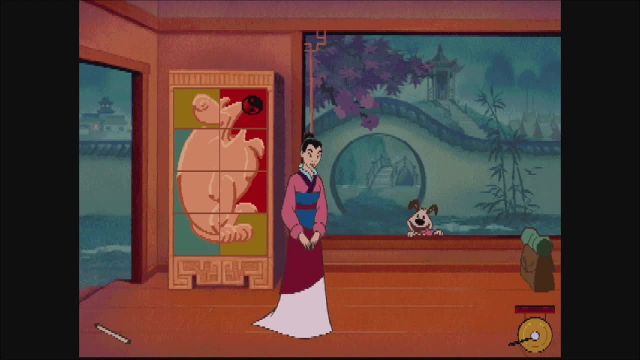 or to go battle with the Huns. All three of those words technically work for the context of the movie, So I don't know. It feels like they should have had like more distinct words rather than words that basically boil down to the same thing. 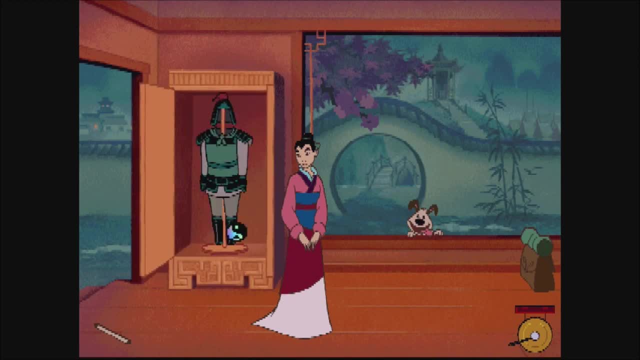 There you go, Anyway. so what year did this game come out? 1998.. The same as the movie. Only a couple of the storybook titles were out of sync as well. Only a couple of the titles were these storybook titles. 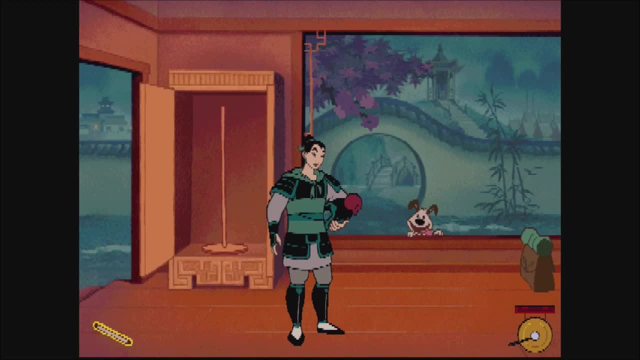 were out of sync with your John movies. All right then. All right then. After finishing both this game and the storybook stuff, Disney Animation Florida went on to make better pair. Go on. In that case, my best bet is that the Game Boy Color game. 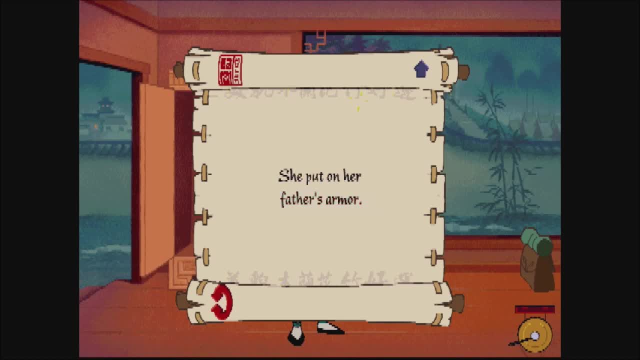 was meant to be the action game, whereas this would be, of course, the storybook game. I guess I never. I was never really aware of the Game Boy Color game when I was growing up, so I guess I completely skipped that one. So 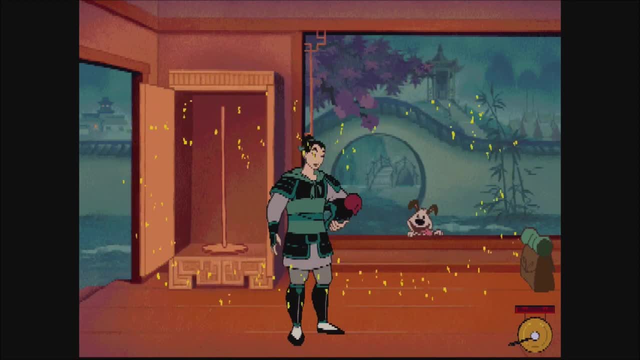 but hey, look at the bright side Turns out Mulan did get an action game after all. Oh yeah, that's cool. I just wish it would have been on consoles, like the other ones. Yeah, honestly, I do agree, At the very least, 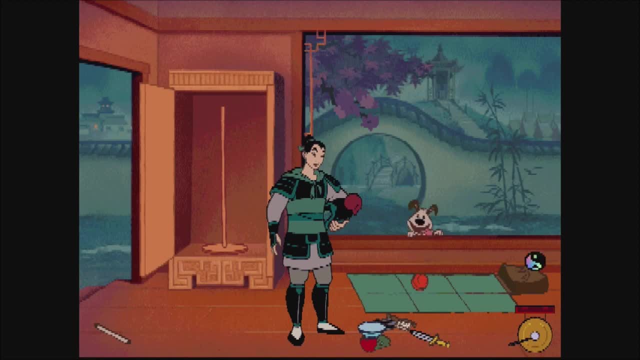 like it feels odd to be the one kind of sticking out compared to Hercules, you know, and seminar. I suppose that is a good point on the. on the other hand, I wouldn't necessarily scuff at a game just because it's on handheld. 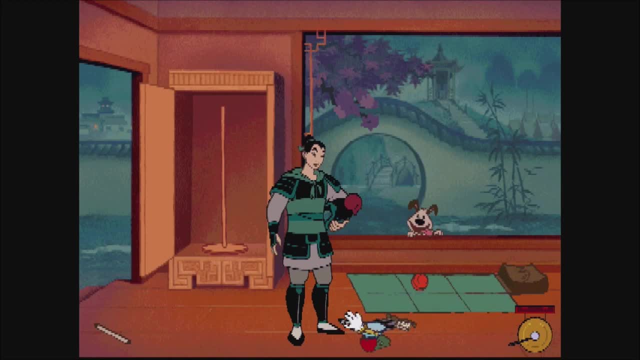 like sometimes handheld experiences could trump even the console ones. Oh no, I'm not saying the game is bad because it's on handheld. I'm just saying like I was expecting at the time a game, they would either use the sprite, animation. 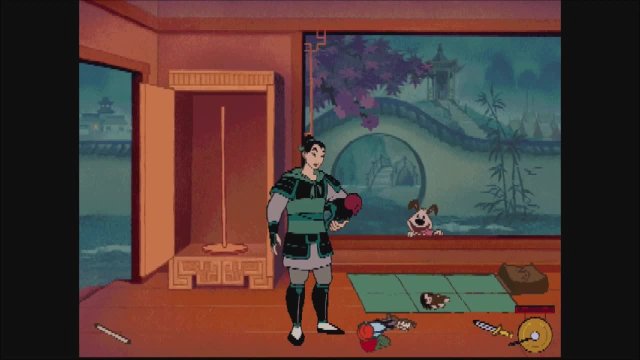 like this game, like Aladdin did, or a game like Simba's Mighty Adventure, where it's a 3D game with clips from the movie. you know, which is what was the norm that they were making back then, you know. 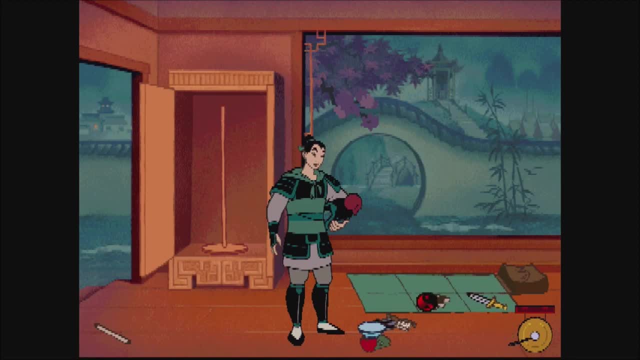 but we never got a Mulan game like Simba's Mighty Adventure. In regards to the team that normally did Disney console games, were they the same one who did this? No, this was made by New Kid Co. the same developer that made the other. 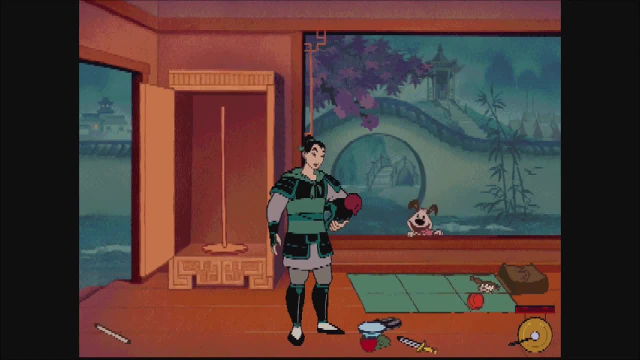 storybook Disney games. They were a completely different developer. Remember, they're a PC developer. So is it possible that the team who usually do the Disney action games were busy with something else and that's why we didn't get a console one for Mulan? 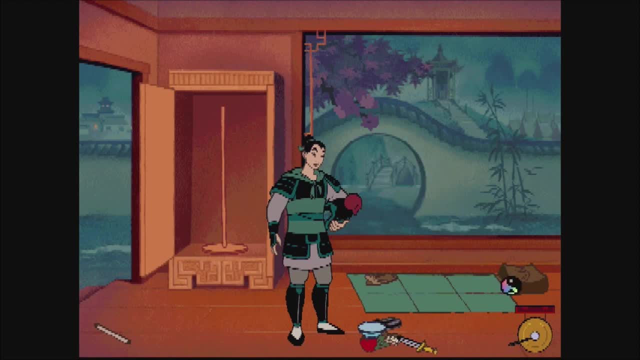 Actually New Kid's Call or Kid's Revolution. the statistical revolution of software was only possible for the PlayStation port. The main developer for the PC version was just the Disney Interactive, with just a couple of minor associations like Media Station or Creative Capers. 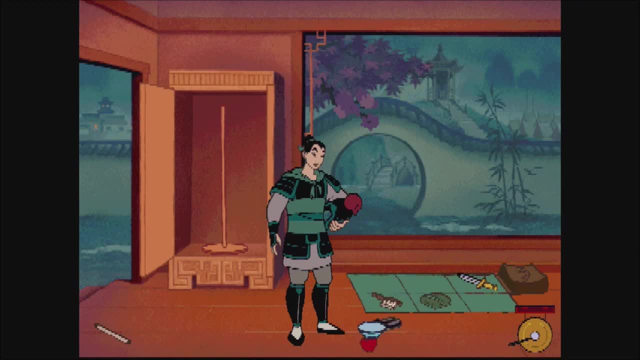 Well, whatever, okay, so I know. Well, that actually still works, Jovo, because remember most of the other. for example, the Lion King game, Simba's Mighty Adventure was developed by Paradox Development. Disney tried to publish it. yes, but technically they didn't develop it. I think it was the same. okay, if I remember correctly, who developed Hercules? Oh, Eurocom. Eurocom developed Hercules. So most of the games on the PS1 by Disney weren't actually developed. 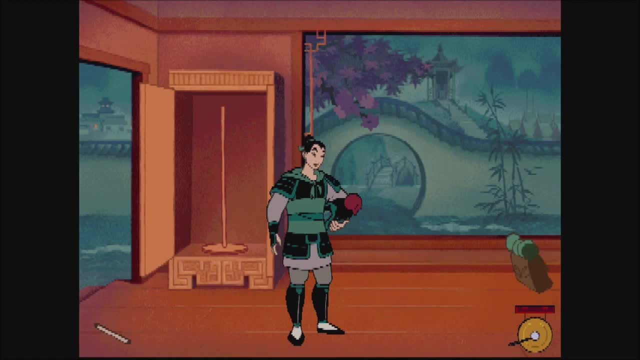 internally by Disney Interactive. so, according to what Theo just said, it seems like Disney Interactive developed the storybook once. So Oh, that was a pretty big jingle there. Yeah, But yeah. now my best guess is that the reason we didn't 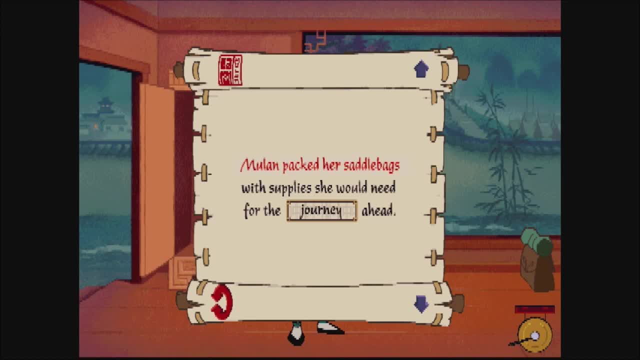 get a console for Mulan an action game, was because they probably couldn't find whatever team they thought would fit best for it. Again, that's just my best guess. Okay, can I voice a complaint about these scrolls They always have. 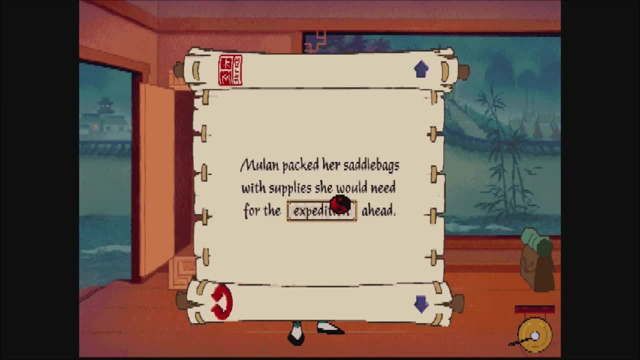 the correct word to use as your first choice. I'm not kidding. You don't even have to actually attempt to decipher the word. I'm not kidding. The word that is the right one is always the one that's already there by default. 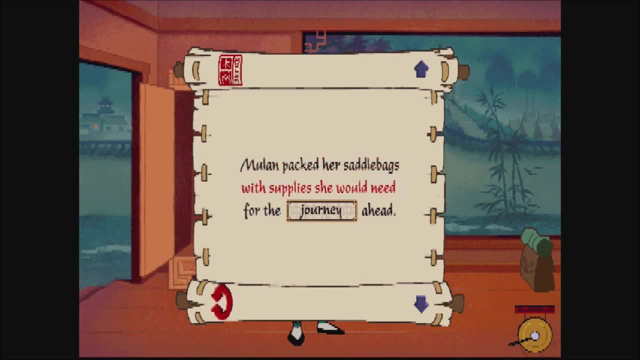 So you don't even have to actually do anything, You can just immediately skip to the. The reason you're not I'm not doing this is because I want you guys to actually listen to this shit. But Go to 27 minutes or something. 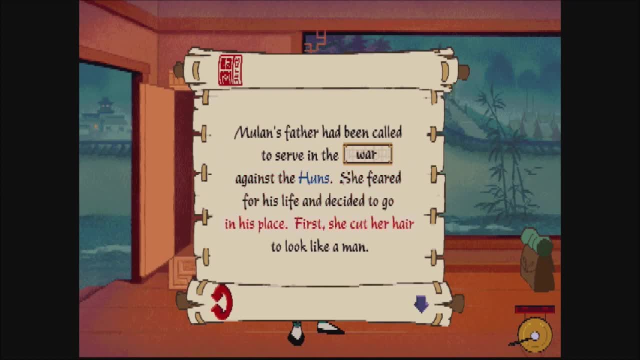 But yeah, that's basically it. You don't actually have to think to do the scroll swings. Yes, To do the scroll swings, because the word they're looking for is already the one that's already there by default. I mean, come on, guys. 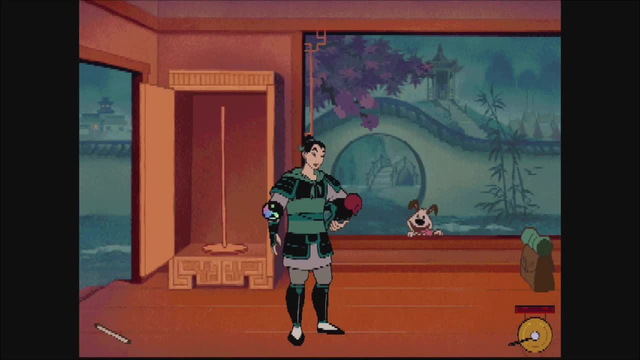 I get that this is for preschoolers, but can't you at the very least ask them to, at the very least, give a slight bit of a thought into the puzzle? Come on Like, Especially because, as the psychologist will tell you, kids hate being. 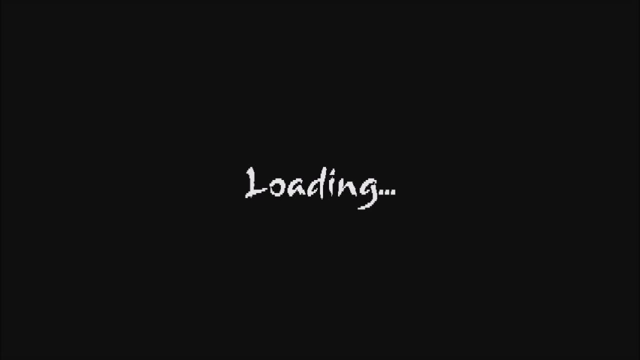 talked down to. But anyway, All right, I wouldn't say it was a bout of them talking down to kids. It's not like they automatically tell you it's gonna be the first one. Click, There you go. Go on, Jova. 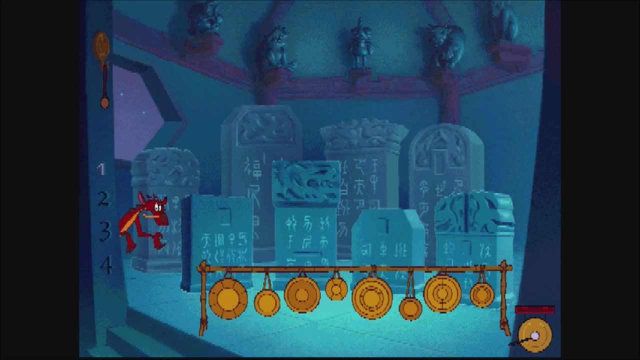 It's not even a case where they automatically tell you it's gonna be the first one. It's more so for the kids to figure out there. I guess it's more like a pattern that you could pick up on, Like I've seen bouts. 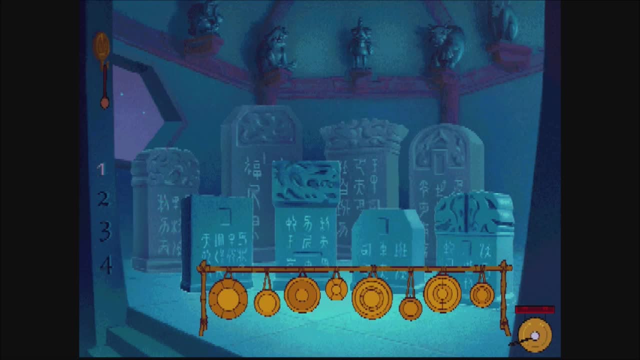 where they do talk down to kids, I would not say this is one of them. It's just more so about what they didn't think to have this or that, And for a kid who's just learning vocabulary, which this game was probably aimed- 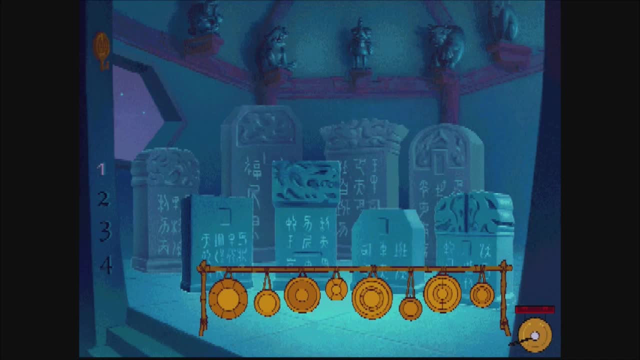 towards. it's fine, It's something along the lines of the Reader Rabbit series. I'd say, Sure, All right. So All right, Let's try. You know what they could've done, though Do something like the. 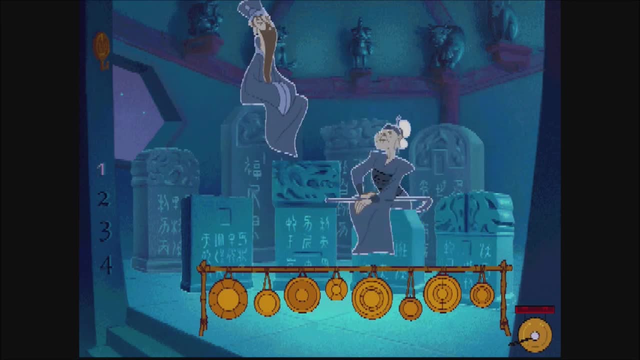 Tarzan CD games, where sure, you got some storybook elements, but you've got different games to do for different start, different segments. There's also the other thing that playing a game like this with a controller rather than a mouse. 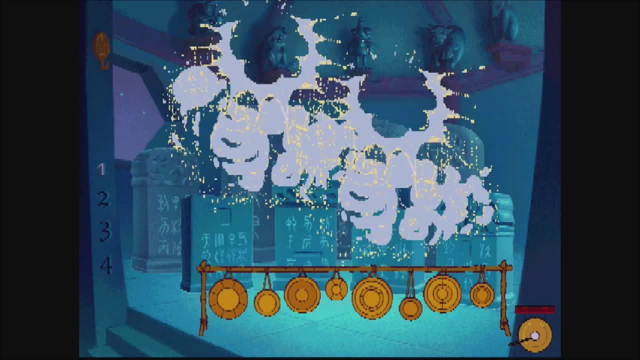 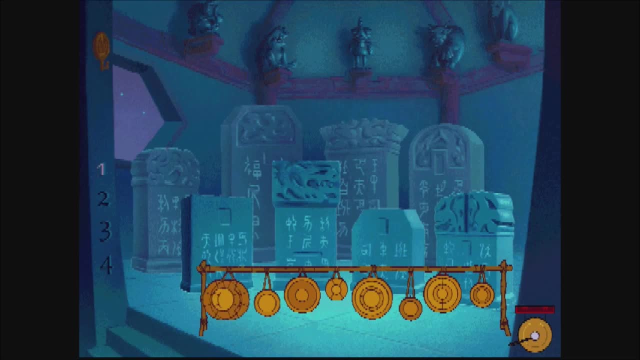 it's not quite as intuitive for me, because when it comes to using a cursor like this, I definitely prefer to use a mouse, which I mean. was this game compatible with the PlayStation Mouse too? Do you know about that? Could be. 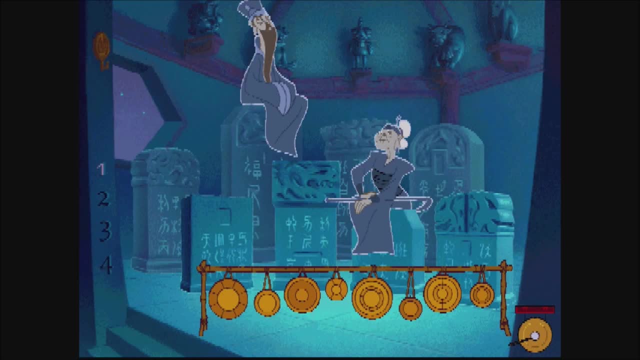 For all I know. Oh my God, That was a thing. That is a thing, Joe. Well, to be fair, Joe most more in Japan than even the rest of the world, but there were a couple of point-and-click ports. like the first clock power and the PlayStation Mouse did work on them. I wonder if this was actually just an experiment and why this is the only game that you could port to the PS1.. I guess, Yeah, basically just to gong until all the. 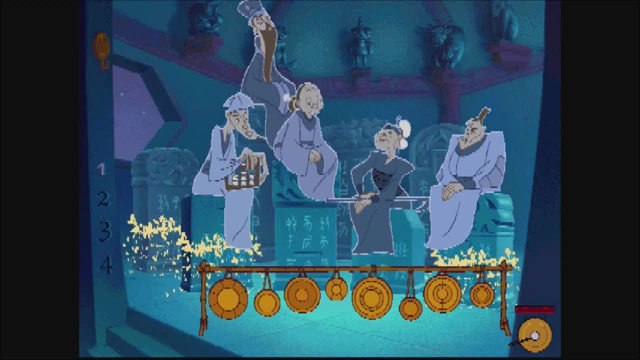 end-testers are back. like There it is. I guess in this version Mulan actually gets to interact with her ancestors. Yeah, basically, Even though this is already. Well, supposedly this is supposed to represent the scene where the ancestors 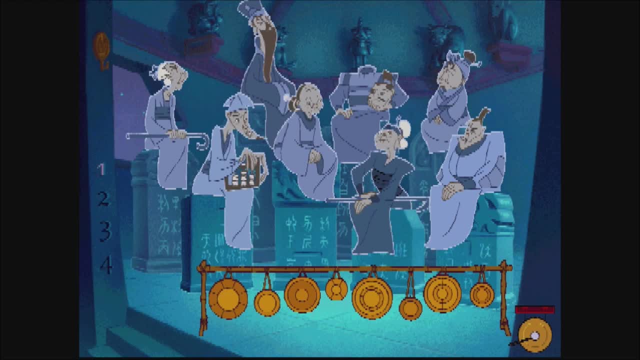 are talking after Mulan departs, Because, remember, we already went through the scene where she gets up her dad's suit and runs away. So this is supposed to be. It's weird, though, because the words by Not Takei in this version. 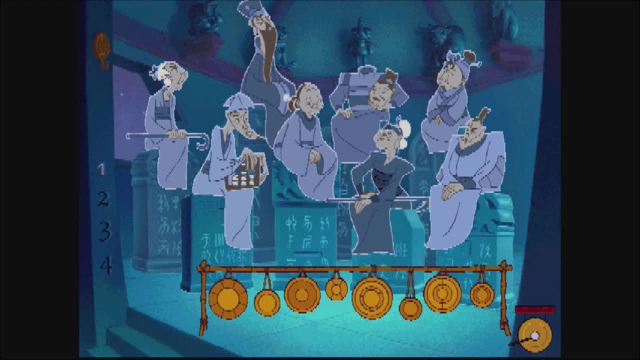 imply that you know that Mulan's the one going to the temple to speak to her ancestors. Well, I don't know what to tell you, Jova. I knew she wouldn't amount to anything. So, Shirai, how long has it been? 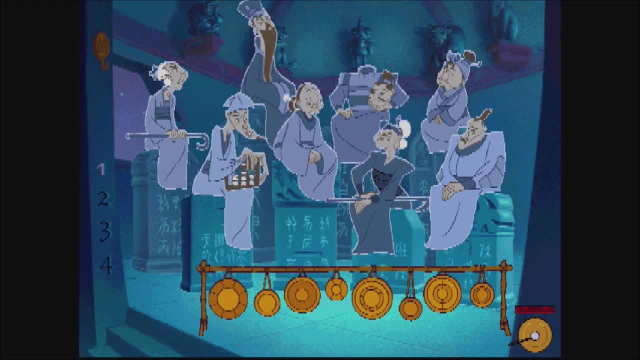 since you played this game A very long time. So what, if Alright, so coming back to it after all these years, like any observations you want to make, I mean it's still cute, and I agree with Jova. 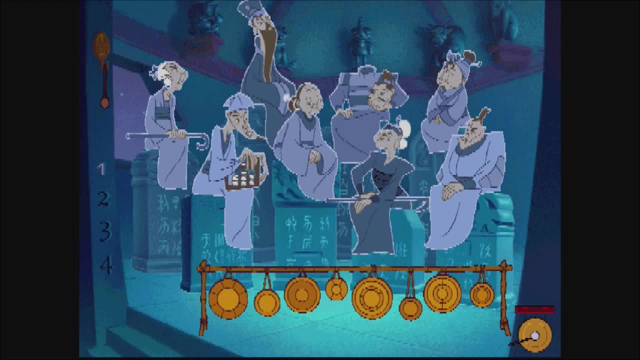 Like it is. You know It's good for you know some audiences, but still don't understand why Mulan didn't get an action game. Mm-hmm, Yeah, like I feel like this about this game. 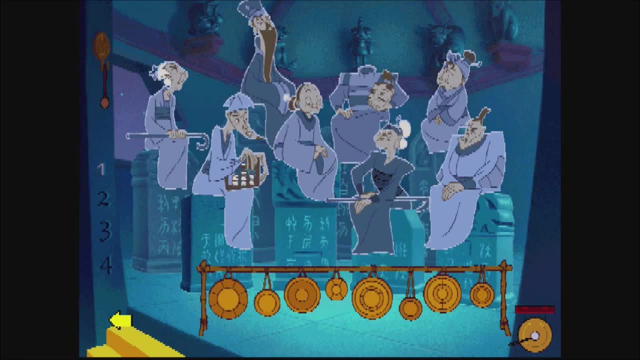 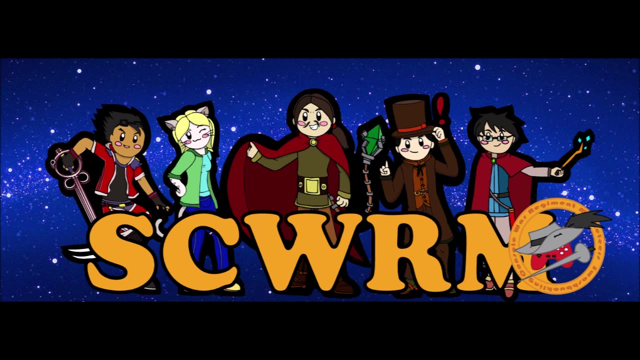 It is what it is for its age- demographic- and I just don't see the point in getting mad at it for this. Oh no, I'm not mad at it, It's just that I've always wanted a game where I would tickle down a ship, you know. 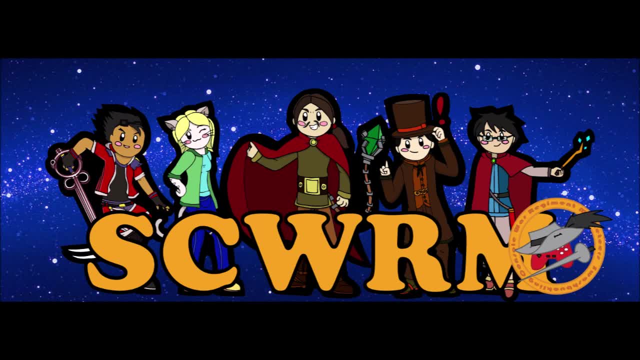 to shun you in a boss spell, and I had to wait for Kingdom Hearts 2 to give me that. you know. Yeah, I think it's kind of like a similar sentiment that Castlevania fans had when the Lords of Shadow games came out. 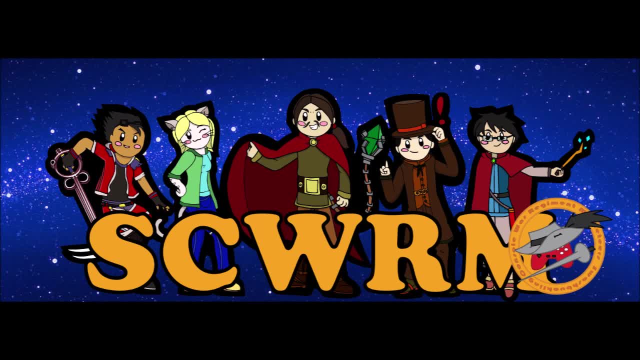 It was not necessarily for what they were on their own, but because they were just present only then and nothing, and they may see it was not continuing as they wanted. I think if it was a case where a proper game co-existed with this one. 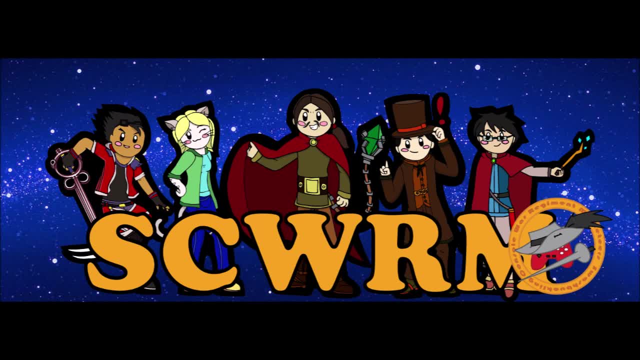 this one would not be that much. you know, looking this light. Oh yeah, definitely. There was the Game Boy Color game. Oh yeah, I get that, Jova, but I still think it would have been even better to have that. 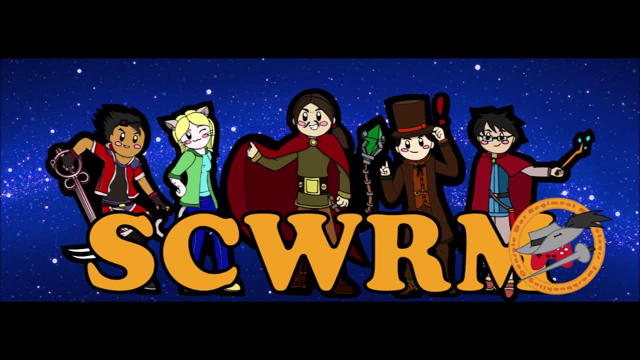 this game and an awesome Simba's Mighty Adventure type game. Like, have all three of them. Like why stop at two, Let's have three, you know? Oh, I definitely agree with that. It's just like well. 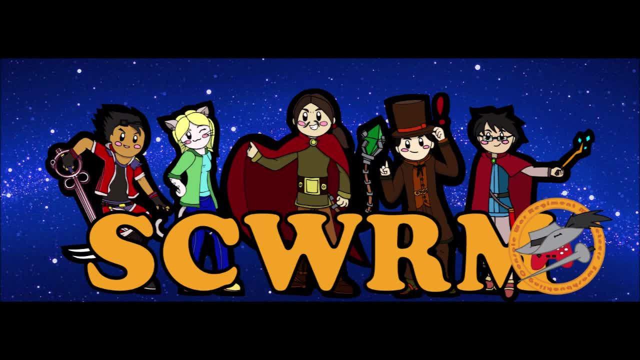 I guess I don't really agree with the idea that we didn't have a proper action game with that. Granted, I haven't seen the Game Boy Color game yet, so for all I know, maybe it was crap or whatnot. I mean, I just hesitate to say.